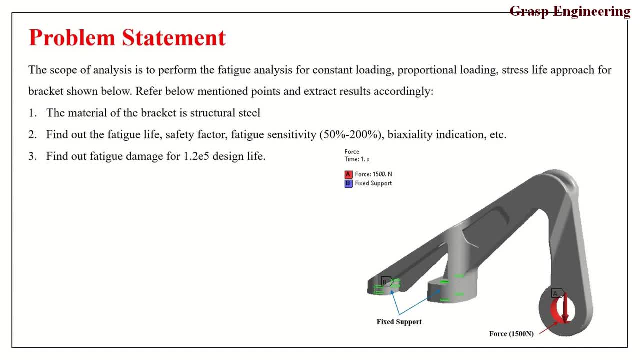 And you will find that it is the force is like 1500 Newton- which is acting downward And it is fixed for highlighted green surfaces in all degrees of freedom. So here, while doing simulation, we need to refer below mentioned points and extract the results accordingly. 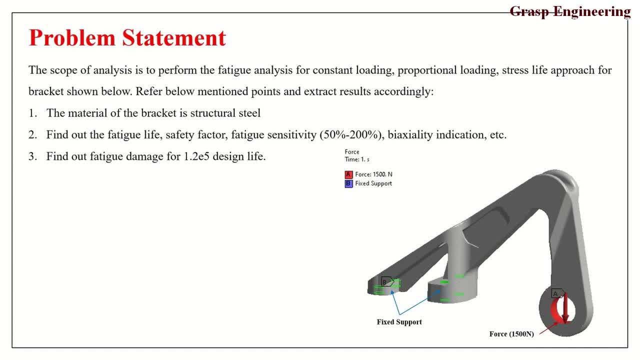 So first of all, we need to perform static analysis. First point is like material is structural steel. Second, we need to find out the life safety factor: sensitivity, biaxiality indication. And third, we need to find out the fatigue damage. for 1.2 e raised to 5, design life. 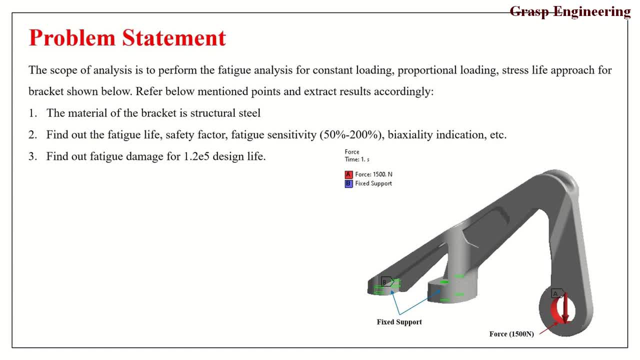 So here you might not aware of what is fatigue life safety factor? what is fatigue sensitivity biaxiality indication? So what we can do now, we will go to our Ansys, our blog, where we explain all these terminologies. 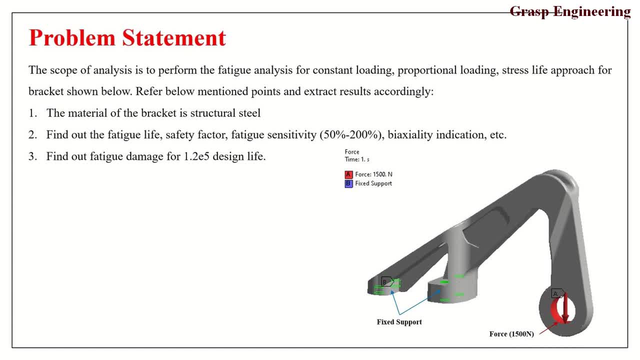 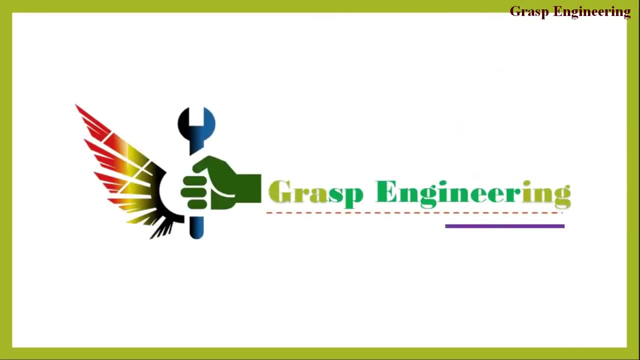 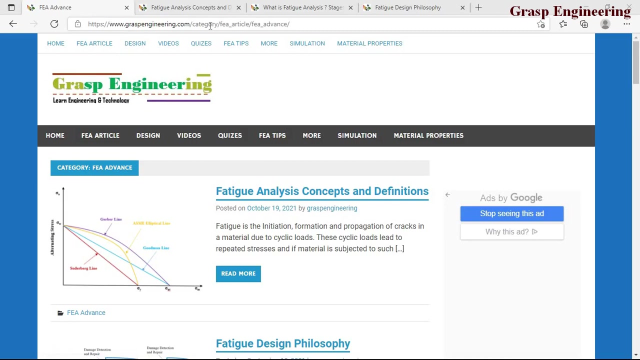 We will go through that And then later on we will go to our actual simulation part, like how to perform fatigue simulation for this applied loading and boundary condition. We are inside our blog post, that is wwwgraphsengineeringcom, So inside this blog post you will find the variables. 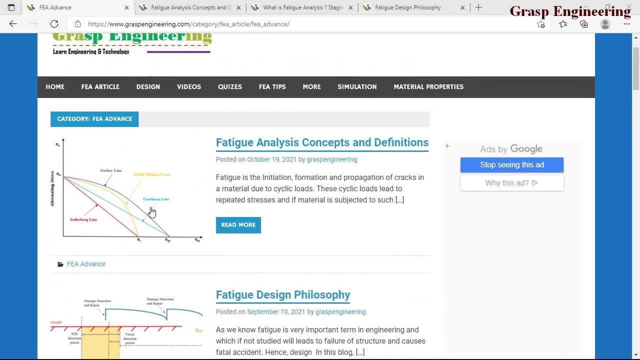 You will find the various concepts explained which are related to finite element analysis as well as design. We also explain few quizzes, like FA square quiz, as well, as you will find few tips, And then we also started uploading the material details, And you can also find out the FA CAD geometries for your practices from here. 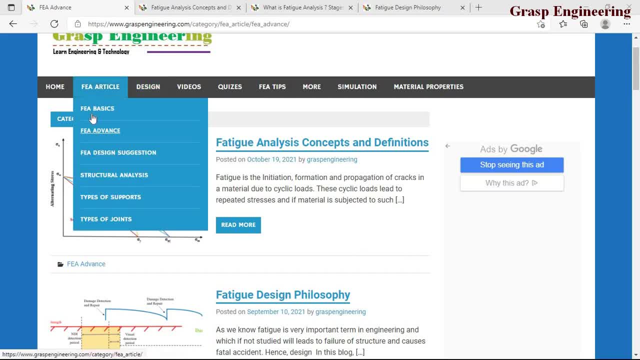 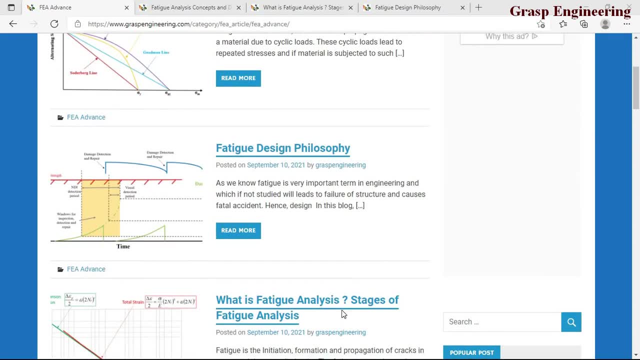 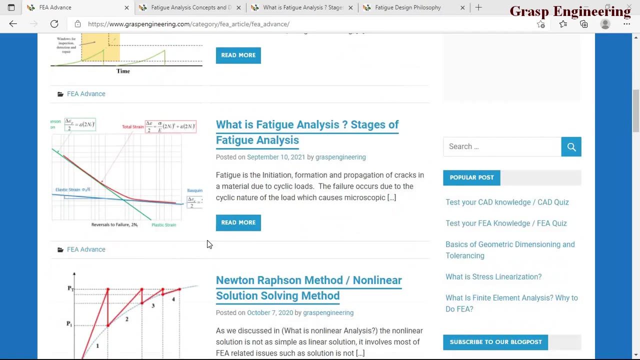 So let's move to our present topic, that is, fatigue simulation. So here inside the fatigue FA advance, you will find various blog post. So now there are, like present, three blog posts which are related to fatigue analysis. So here I will suggest you to go through this, first to explain what is fatigue analysis, to see what is exactly the fatigue analysis. 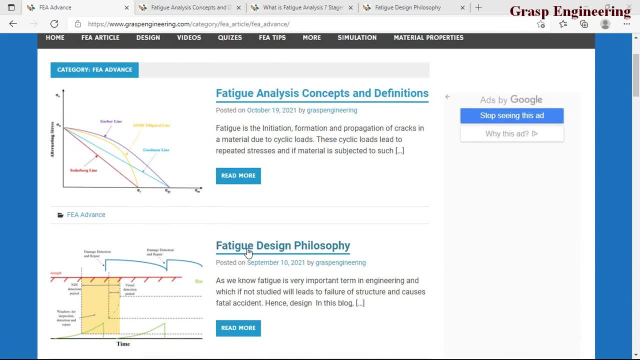 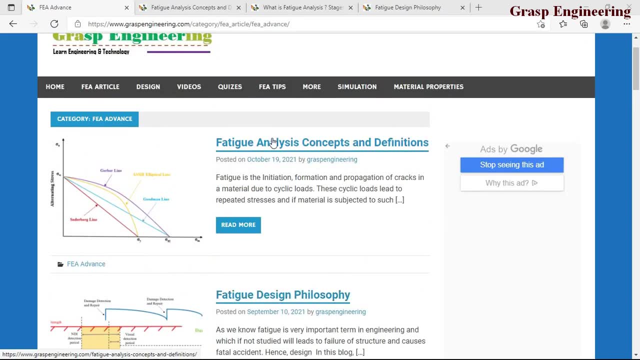 What are the different stages of fatigue analysis And also you can go through the fatigue design philosophies. What are the different philosophies And at present video we will discuss about the. what are the concepts which are useful to perform the fatigue analysis? 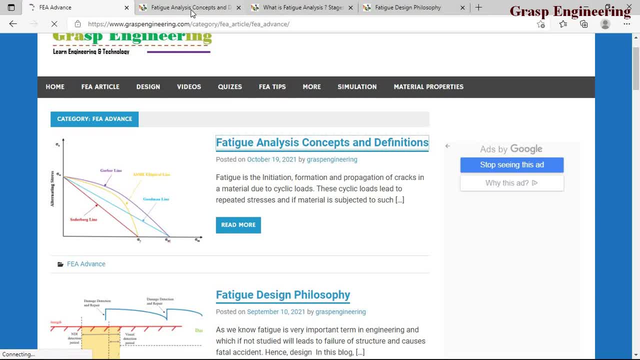 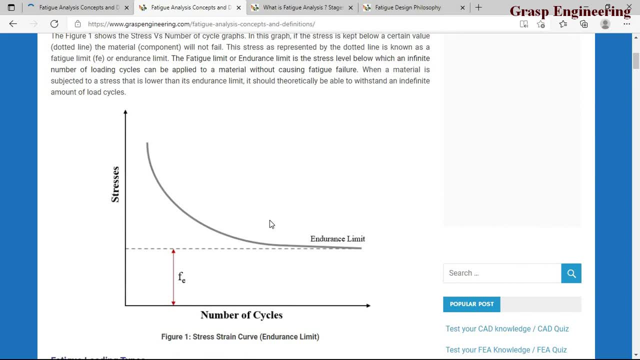 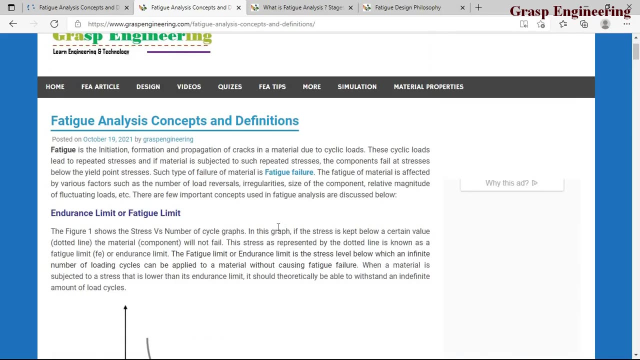 Okay, So if you click inside that, it will take you to this page. So this is what, the page which explain the what are the different terms which are useful to perform your fatigue simulations? Okay, So the term like, as we know that, what is endurance limit, fatigue limit? 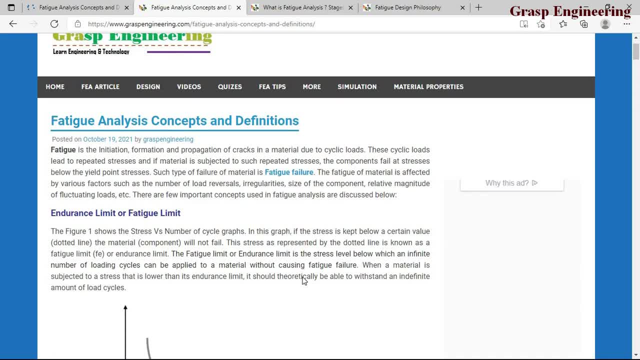 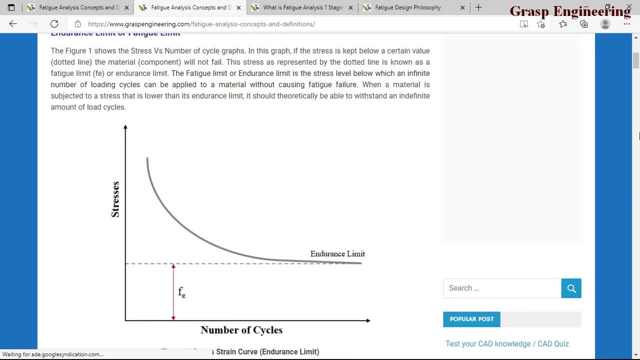 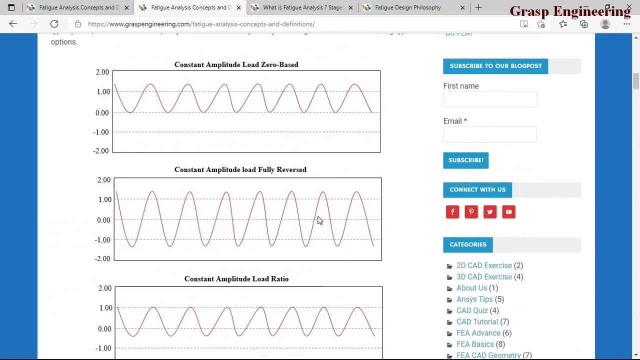 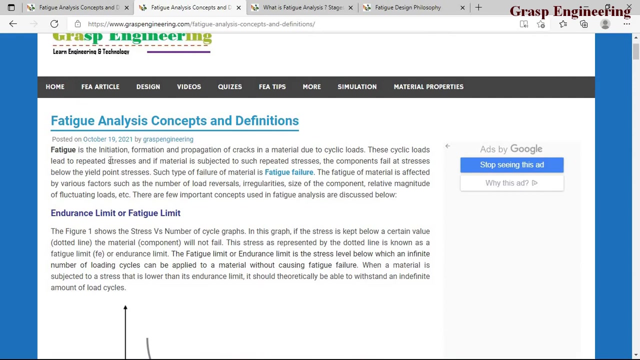 So all these things you will find here, explained with the help of sketches or graphs. So what we can do now we will just see which is useful for us. So now, when we talk about fatigue, so what exactly fatigue means? So fatigue means like initiation, formation and propagation of crack in a material due to fatigue. 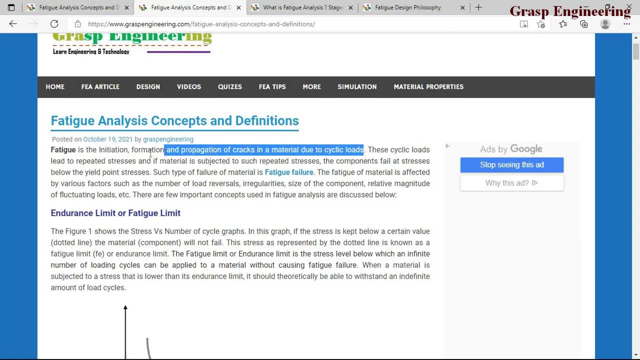 Okay, So this is what we can do now. So fatigue will go down to cyclic loading. I'll be aware of that. When there is a cyclic load, it may lead to alternating stress, And that alternating stress may lead to the initiation, formation and propagation of a crack. 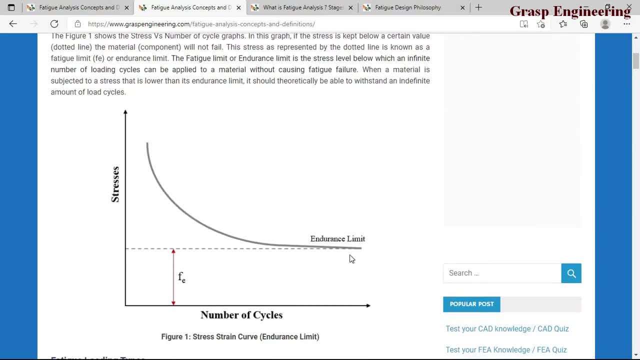 And this graph is nothing but your endurance limit graph. So you can see like this is stress versus number of cycles. When it will go down After this, you will find there is no fatigue failure. so this point is nothing but your endurance limit. so when we talk about 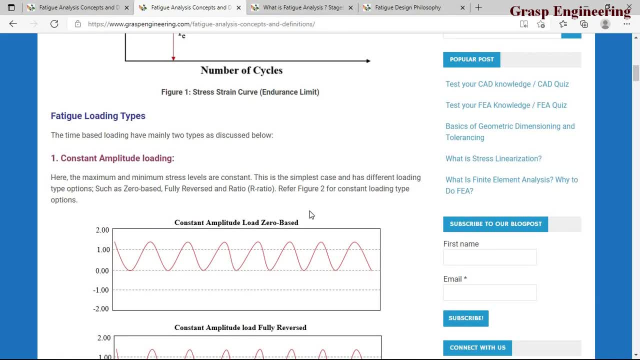 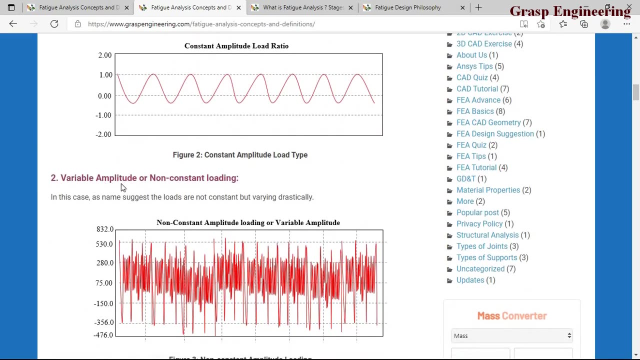 fatigue loading. it is very important term, like when you have a fatigue load, so you should able to understand what kind of fatigue loads are there. so there are two major types of fatigue loading. first is your constant amplitude type and the second one is your variable amplitude or non constant. 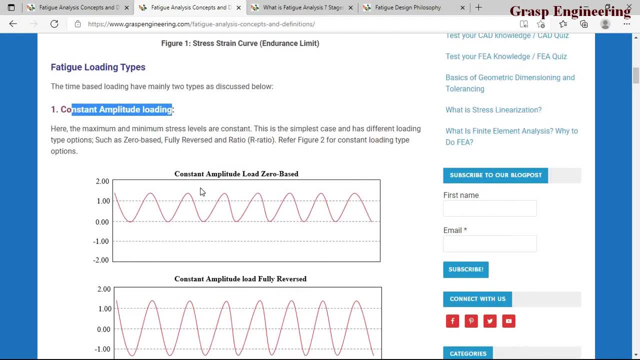 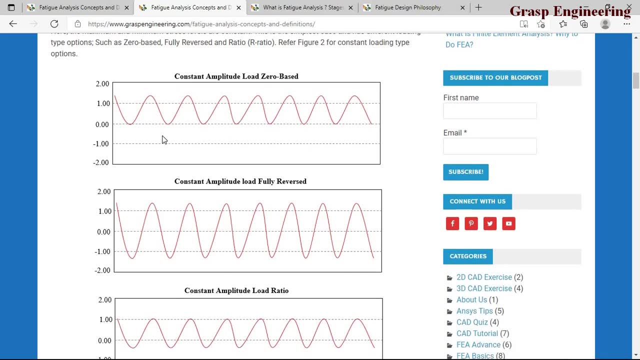 loading. so when we talk about constant loading, it may varies further in three types. first is constant amplitude: load zero, base. so basically, if you see this graph, you will find that it is basically varying from 0 to 1, like this. okay, and when we talk about constant amplitude, fully reverse. in that case you will find: 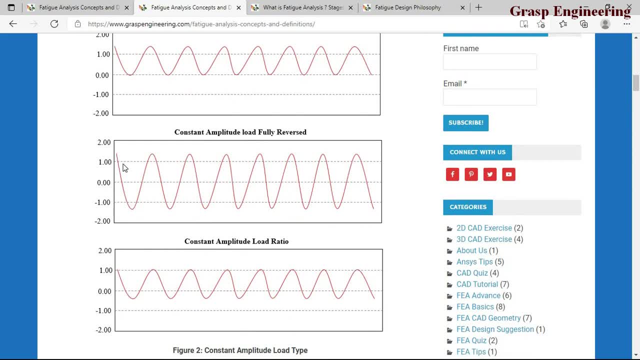 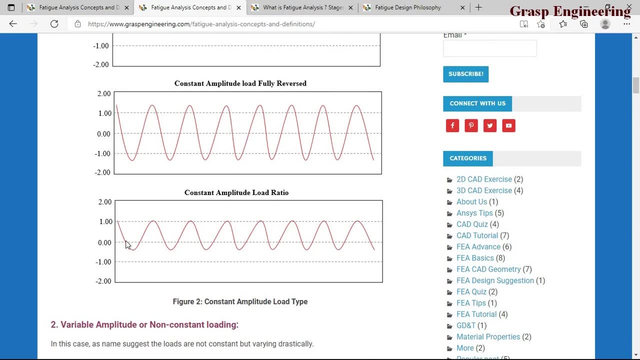 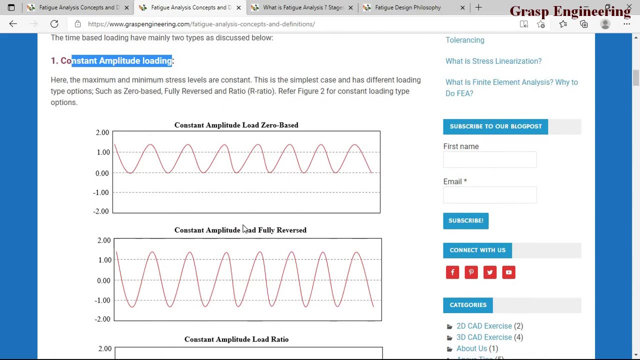 that it is varying from bothi to 1 to minus 1. so, like that, you will find the various peak and valley conditions okay. in the similar fashion, there is a third load case which is, like you can see, like constant studied load ratio. so all these loads, what we can see from this graph, these are: 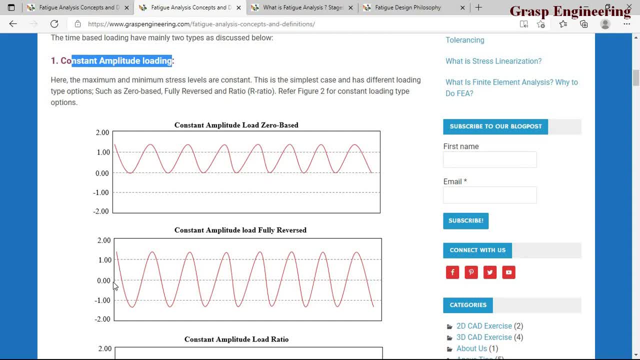 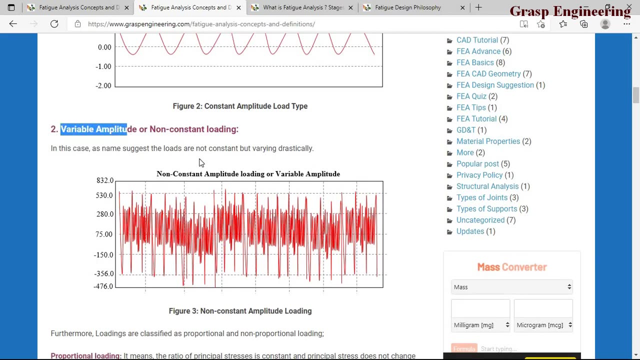 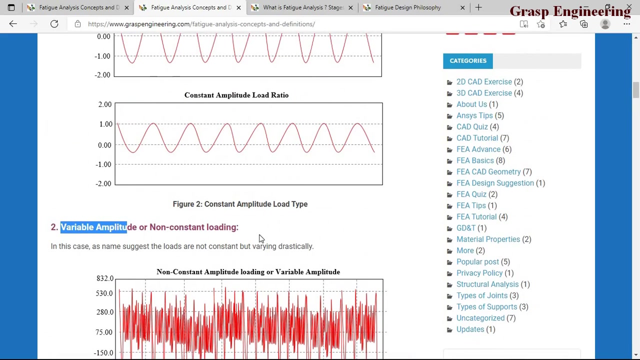 nothing but your constant loading, so which are either wearing positive side or negative side. okay, so when we talk about non constant amplitude side, so you will find that variable or non constant, as name suggests, you will find there is no constant loading, but it may wear, is drastically along this your vertical. 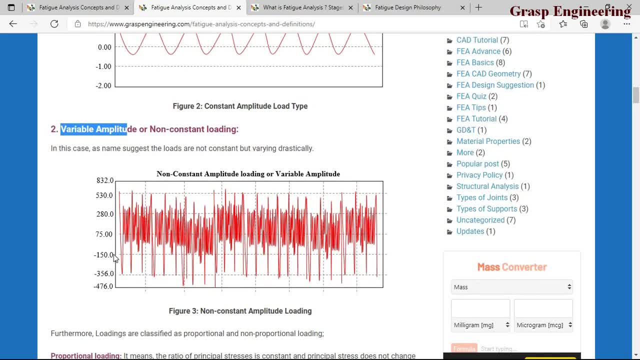 axis. so you can see like you have different values here, like from minus 4028, 32, and it is difficult to predict what is the exact value of this respect to loading cycle. so when you have such a kind of loads you need to refer non constant variable amplitude loading and in real life most of the loads may. 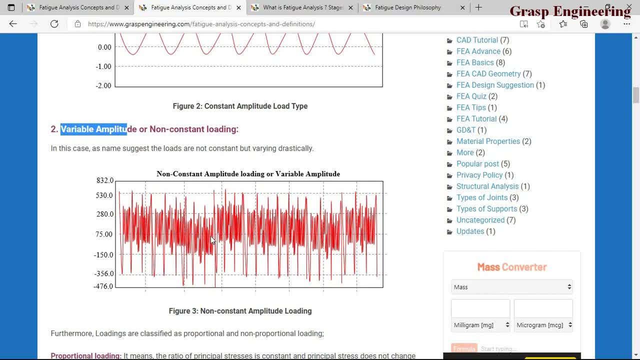 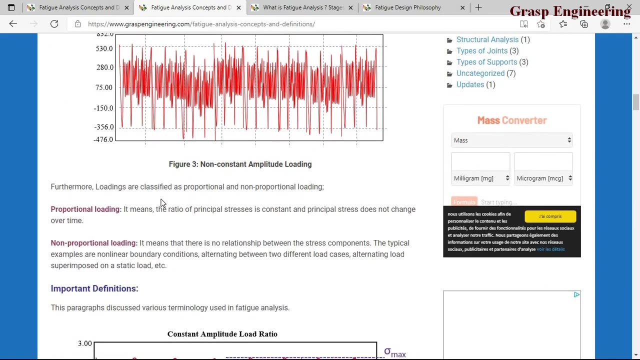 comes under this categories. so while you will going to input this load, you need to select whether it is constant amplitude or variable amplitude load. so accordingly, software will calculate the fatigue life. okay, there are further two more categories like proportional loading, non-proportional loading, so you can just go through that. so I will. 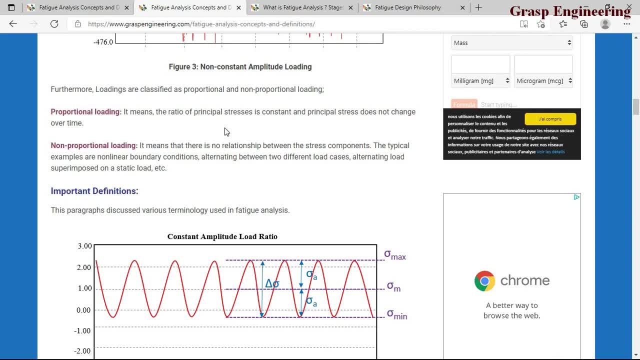 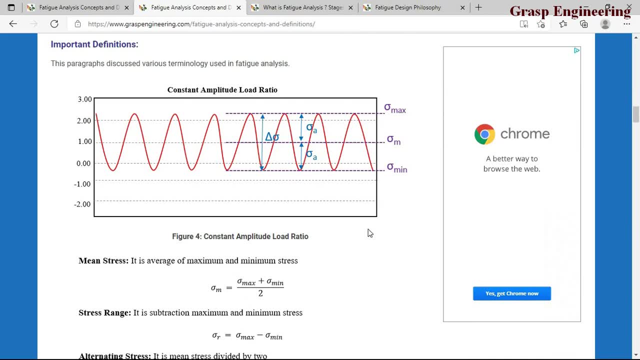 eliminate this for the present video. neither it will take much more time. so let's talk about few important definitions. so I think you already aware what is mean stress. mean stress is basically your maximum minus minimum, sorry, maximum plus minimum divided by 2. so basically it is nothing but the. 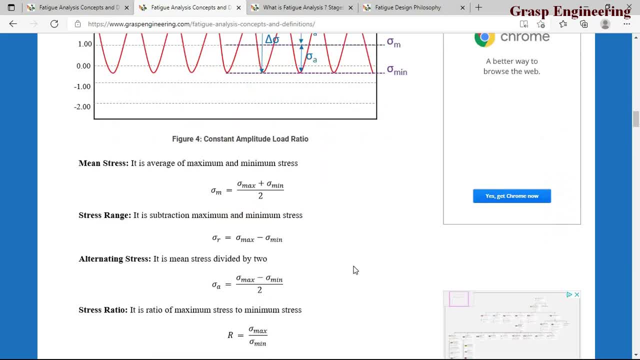 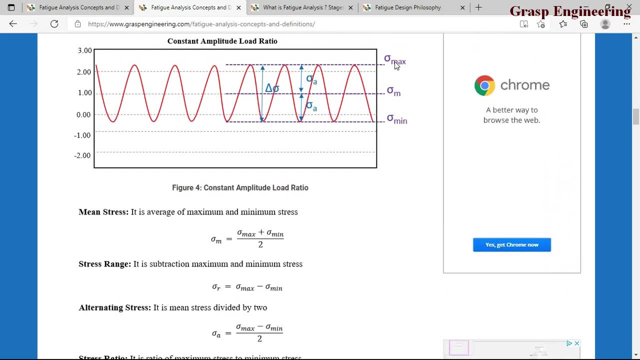 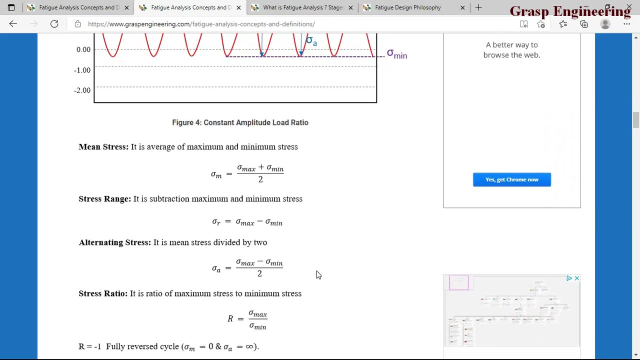 average of your max to minimum. when we talk about stress range, it is like max minus minimum, and when we talk about alternating stress, it is nothing but the average of your maximum minimum. okay, so you can see like Sigma max minus Sigma minimum divided by 2, and similarly there is one more terminology like stress. 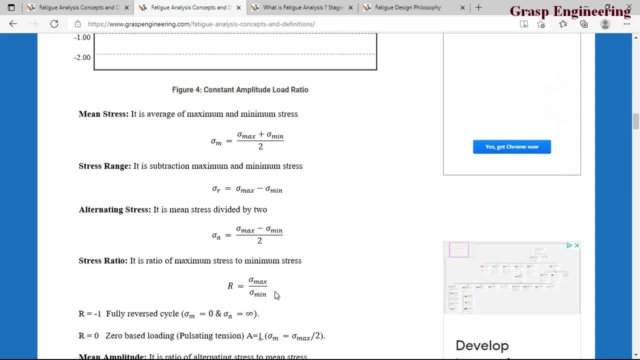 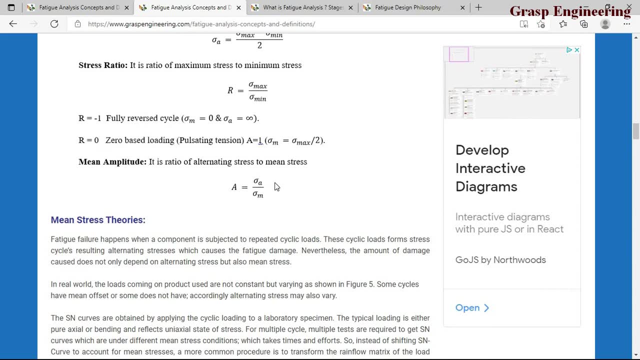 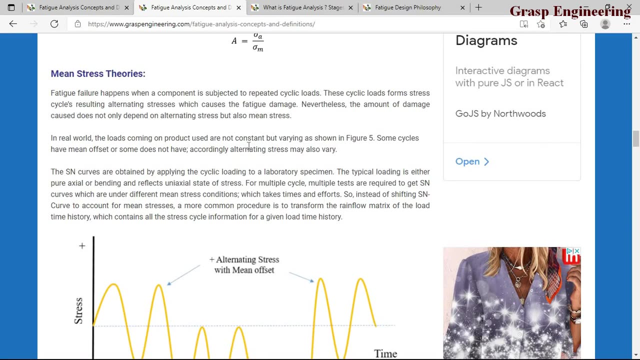 ratio, which is your, nothing but your maximum stress divided by minimum stress. okay, there is one more important term, that is mean amplitude. so it is nothing but the ratio of your alternating stress to the mean stress. okay, now when we do the simulation, at that time it will first ask for your load types and next it will 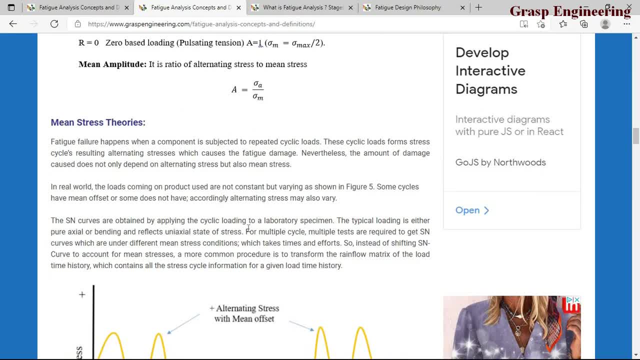 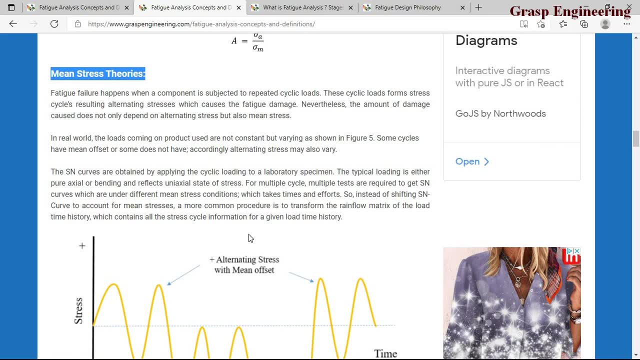 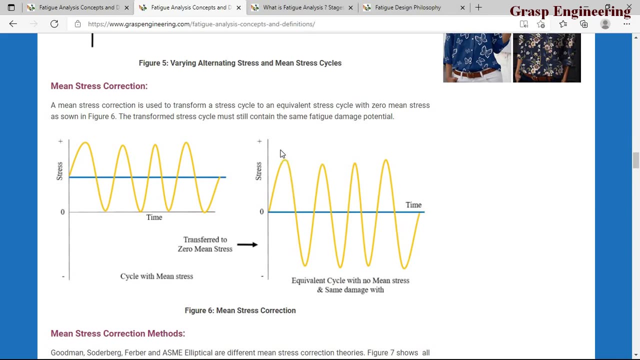 ask for your the respective stary which you need to refer to calculate the mean stresses. okay, so I will suggest you just go through that. I will not explain right now. I mean stress theories. what are the mean stress degrees? so basically, in short, the mean stress correction is not. if you see this graph, you will find that 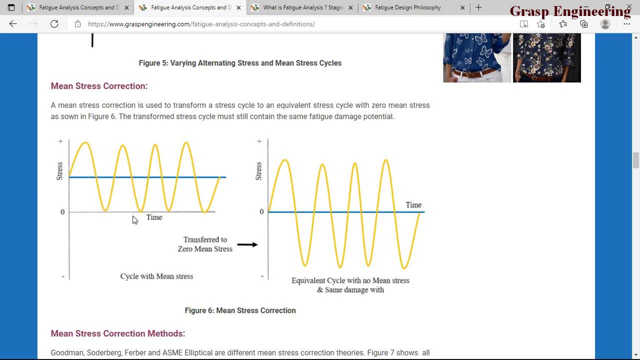 this is nothing, but you will constant loading but it is offset. you can see like: from zero mean it is offsetting. okay, now what the mean stress does mean stress offset. this curve to the equivalent cycle with no mean stress and same damage. you can see like: okay, it got shifted to the 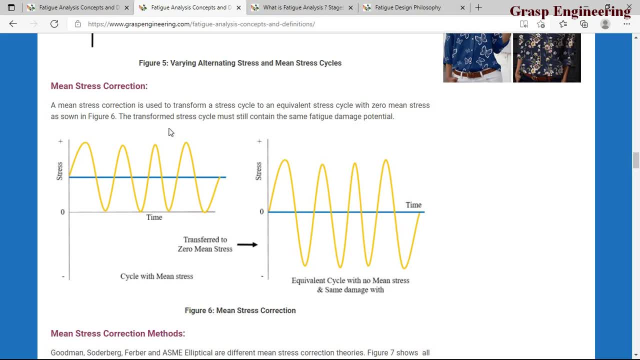 respective cycle, equivalent stress cycle. so here you can see the statement. like mean stress correction is used to transfer a stress cycle to an equivalent stress cycle with zero mean stress, as shown figure below. so here you will find some mean stress value, but here it will get subtracted from max to minimum. so here, basically, you 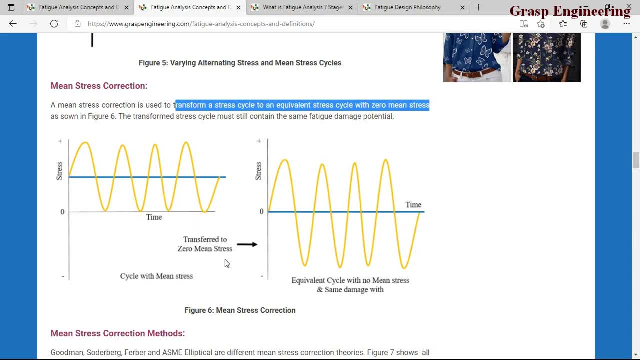 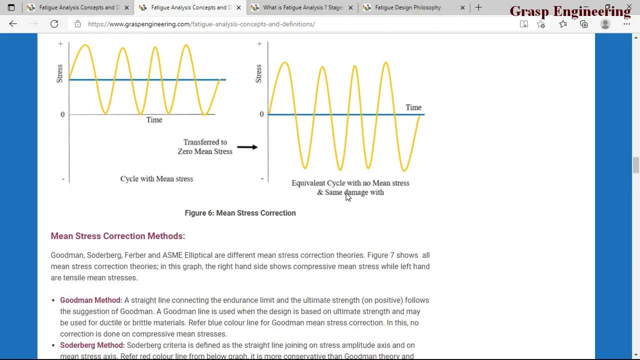 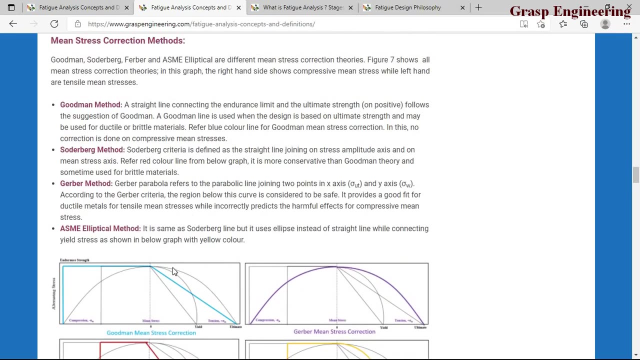 have a zero mean stress, but here you will have some offsets. so mean stress correction helps to transfer this respective cycle to the equivalent cycle. okay, and there are four different mean stress corrections, so you just go through that. what are this? if we have time, we will discuss at the end of this video. so basically the first. 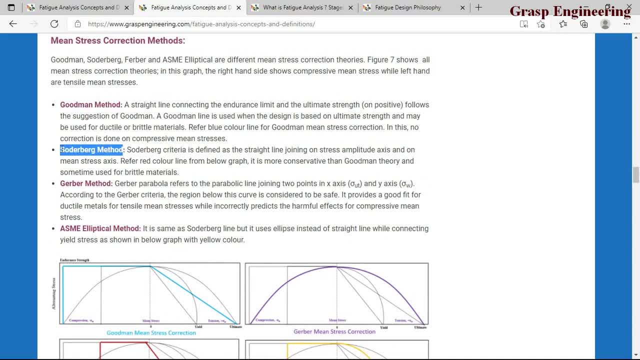 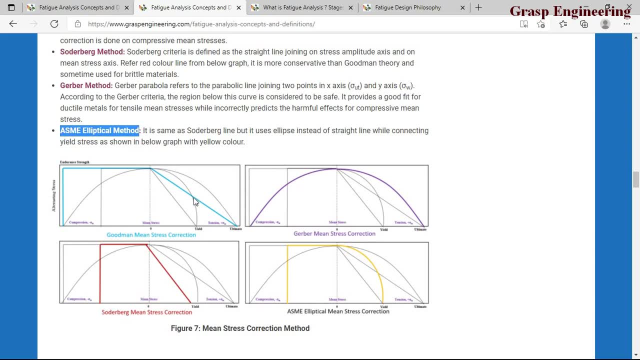 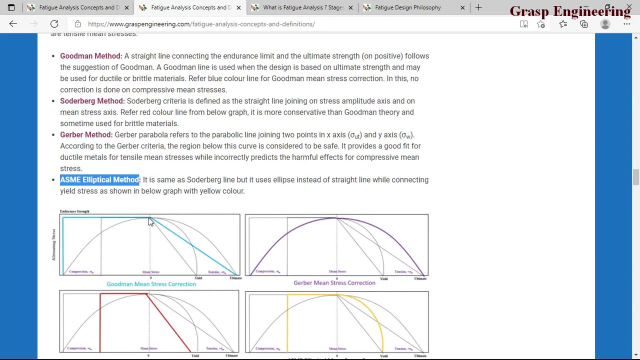 is your goodman method, the second one is your sodalberg method and the third one is: you can see the gerber, and the fourth one is asme elliptical method. in short, the goodman is nothing but when you connect your endurance, stress, value to the ultimate. 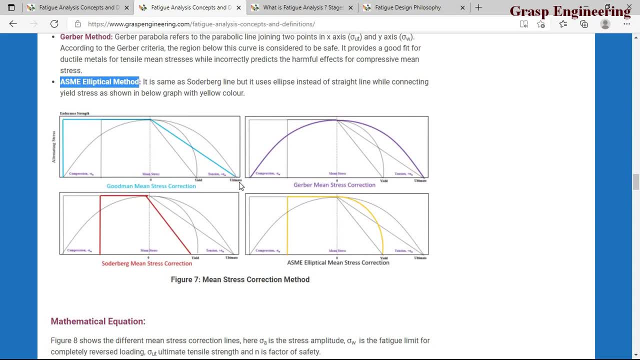 and when we talk about sodalberg, instead of ultimate, you connect to the yield and at the, when we talk about gerber, you will find that this is nothing but the parabolic connections from between the ultimate and your endurance strength and elliptical is as similar to your sodalberg. 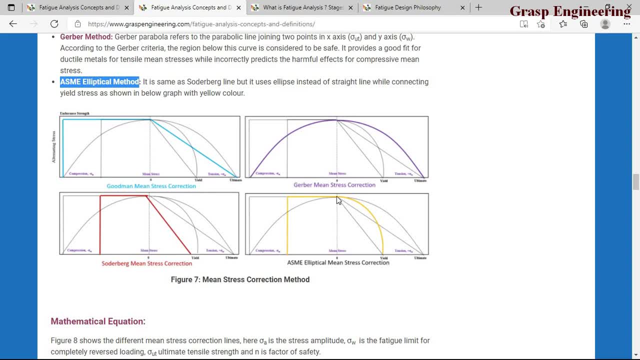 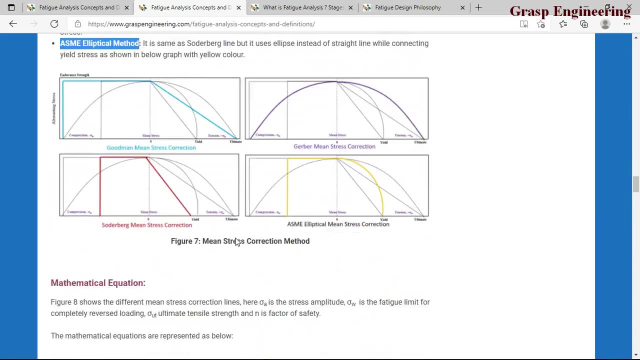 only. the difference between the two is that you can connect the endurance strength and how you can connect the yield to the end strength, and you will find this is nothing but the parabolic nature. you just have a look on this graph blog post. you will come to know what we have written. 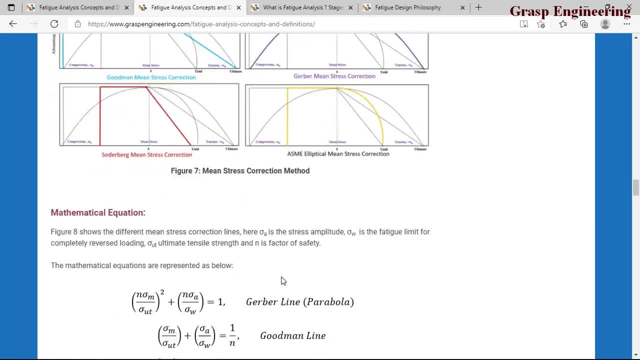 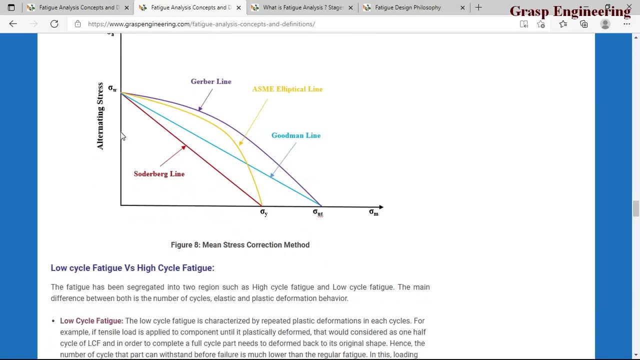 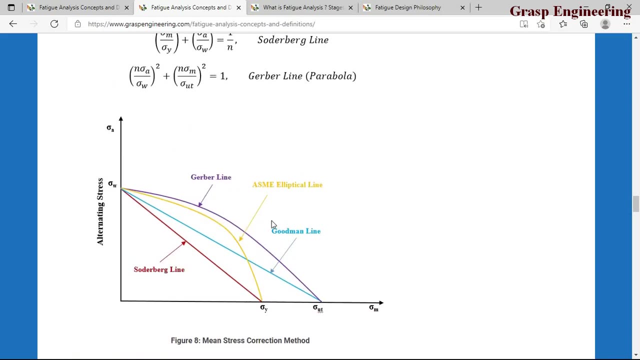 and how this respective values, how this respective theories works. okay, and these are the different formulas which are used for mean stress correction. this is the simplified form of your mean stress correction method. so if you see the difference between difference between this graph and this graph here, this is the compression side. 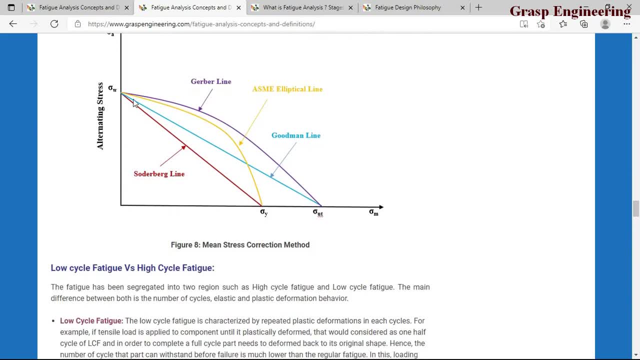 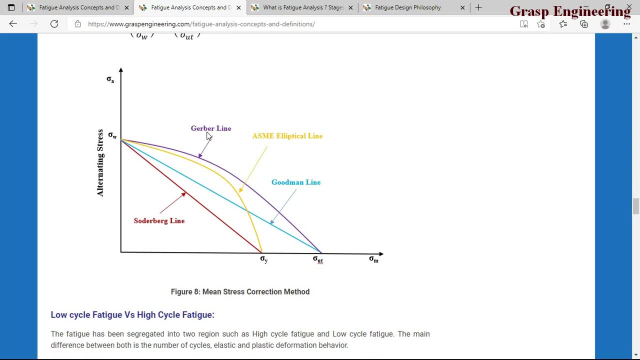 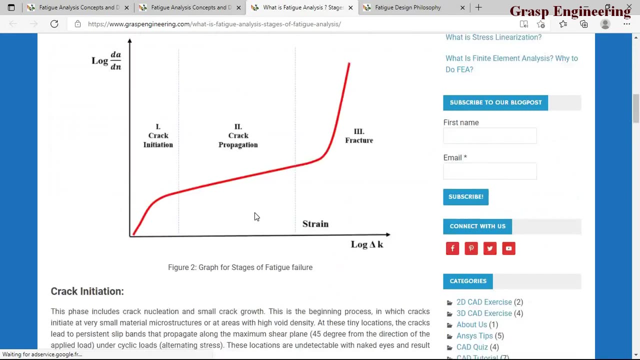 is also given, and here it is the tensile side. so this graph belongs to the tensile side between the alternating stress and your main stress curve. okay, so you just have a look on this. now let's talk about fatigue. okay, this is fatigue, life initiation. so I will suggest you just go through this as well. 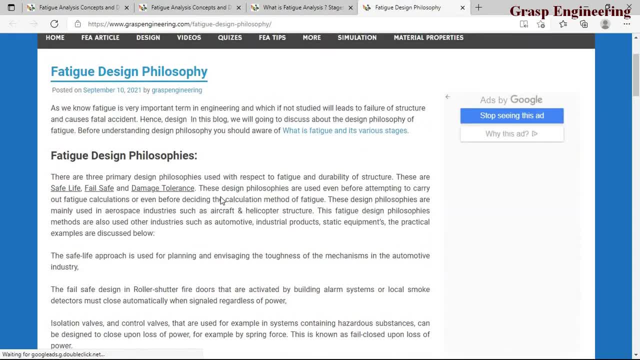 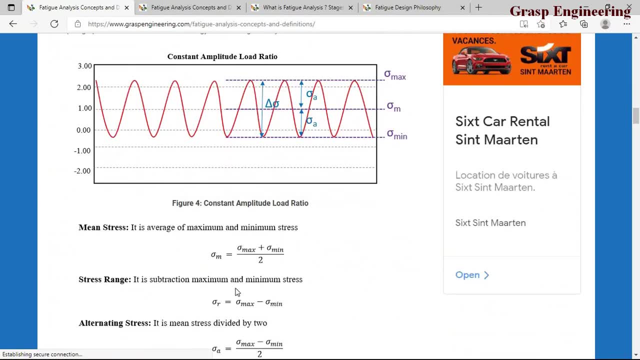 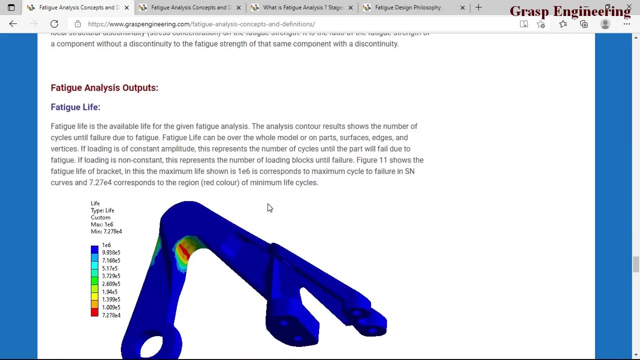 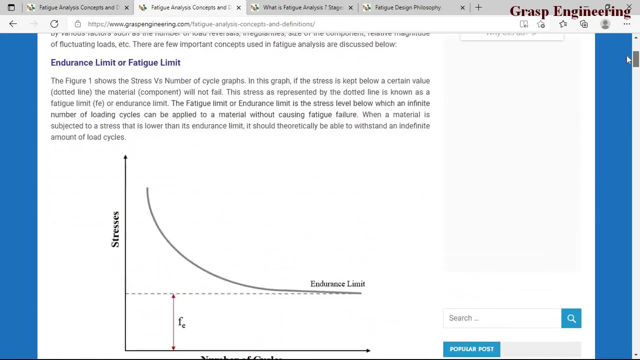 as the what are the different fatigue life approaches? okay, now, when we talk about fatigue, there are two different methods to calculate the fatigue life. so the first one is like stress life approach and another is your strain life approach. okay, so I think you will find that post related to here: fatigue: 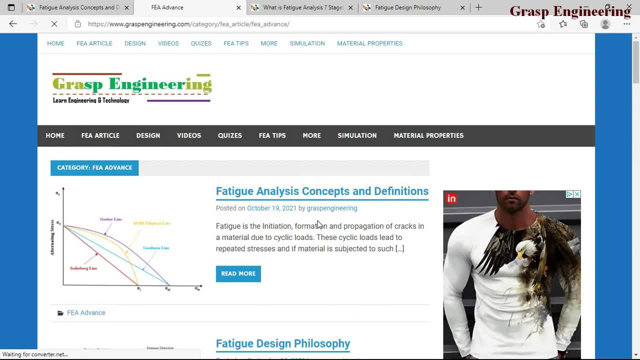 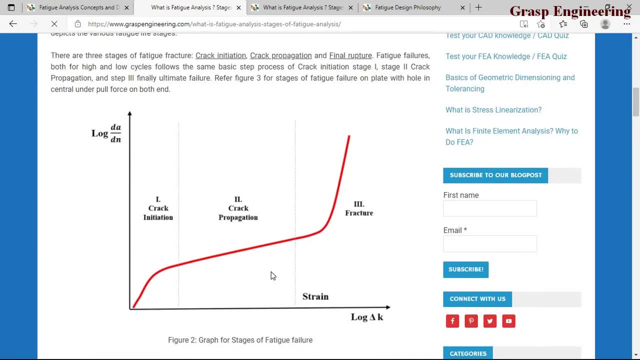 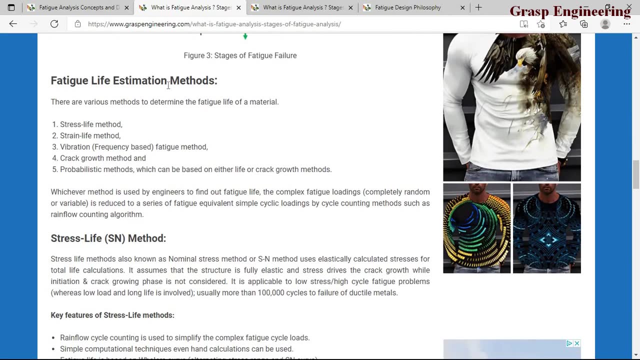 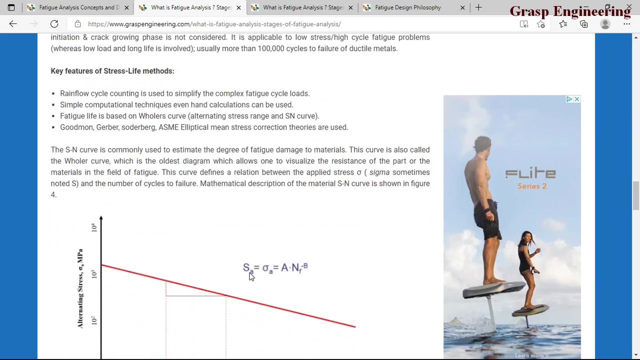 advances. so when you see what is fatigue and stages of analysis, fatigue analysis- you will find here they're like three different stages, like crack initiation, crack propagation and fracture, and then what are the different fatigue life estimation method? you will find the stress life and strain life. so I will 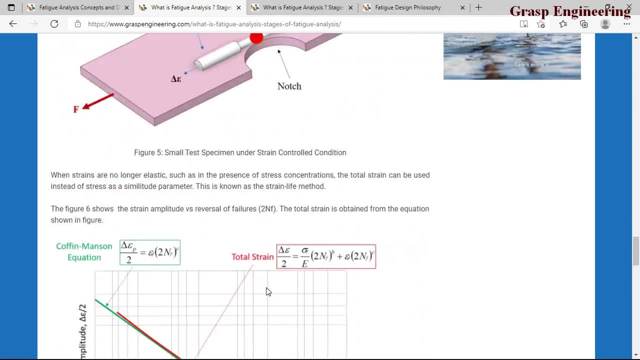 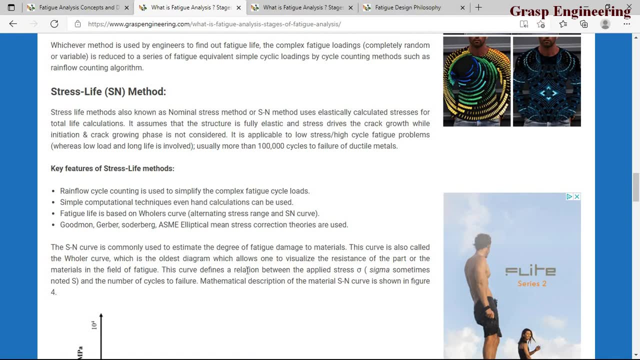 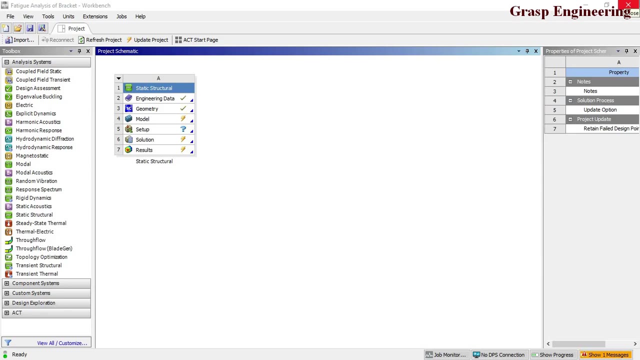 suggest you to go through that. I will not explain right now. okay, now let's move to our actual learning part. so there are answers learning part. so there we will discuss how to perform the answers simulation. so now we are in our actual simulation part, that is answers. so when? 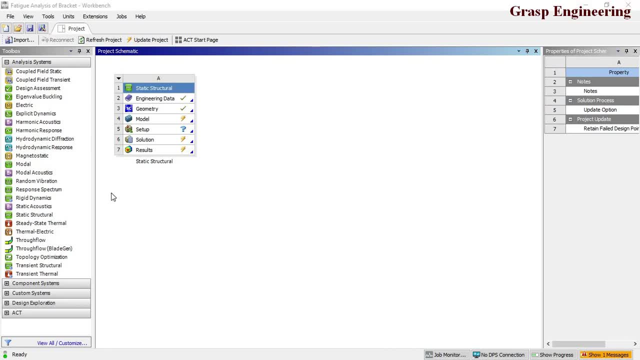 we need to do the FAS simulation. so we just need to refer the analysis system. so at present we are doing the fatigue simulation and before that we need to perform the static simulation. so you just need to drag enter your static simulation in the schematic. so once your static structural 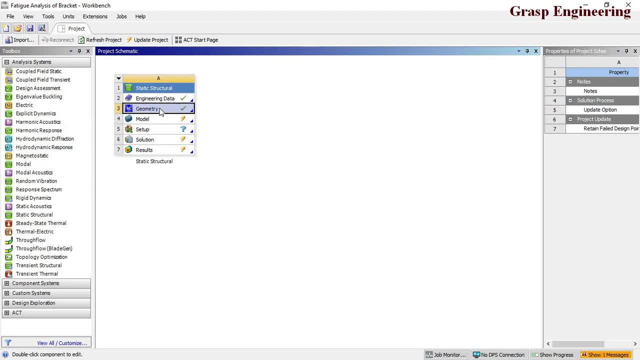 analysis system is present. you just need to right click here and you just go inside the space. claim our design modular, or you can just import your respective geometry from your respective path and once your geometry is imported, you just need to double click into the mechanical to load the geometry under. 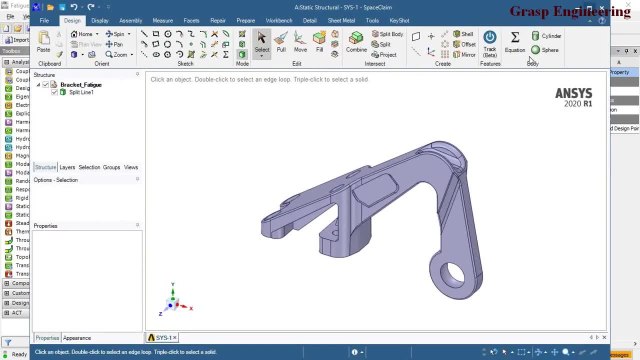 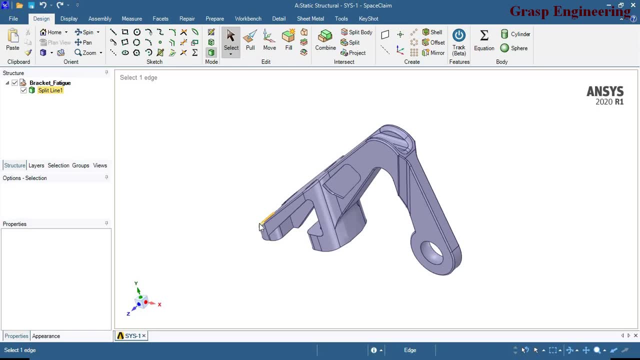 the mechanical. so let's refer to the geometry inside the space claim. so you can see that this is the geometry which we need to refer inside the space claim. okay, so right at present, we will going to use the geometry as it is. we will not going to do any simplification. 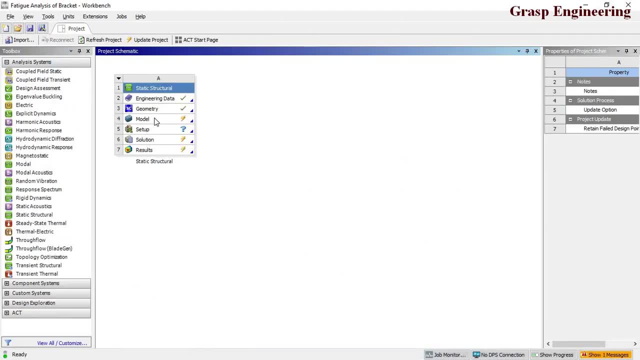 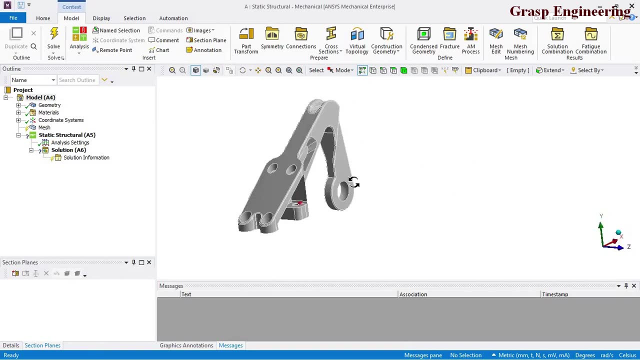 so let's move directly to the mechanical part. so you just need to double click over here. once you will double click, your geometry will open under the mechanical. okay, so now let's start with the simulation. the very first part is to assigning the material. so you can see like here: there is a column called 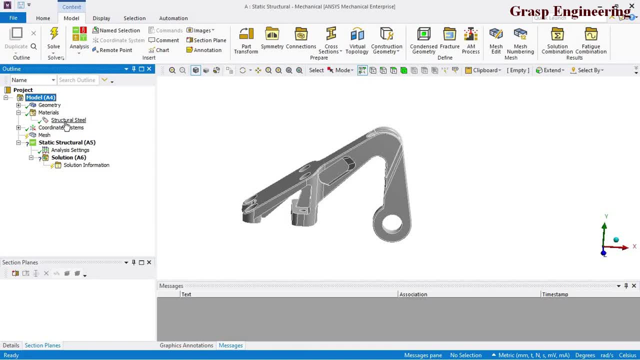 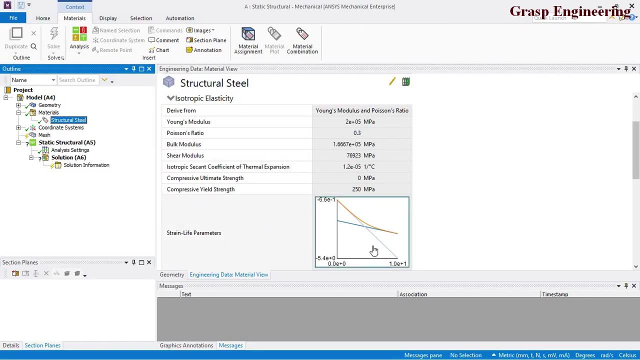 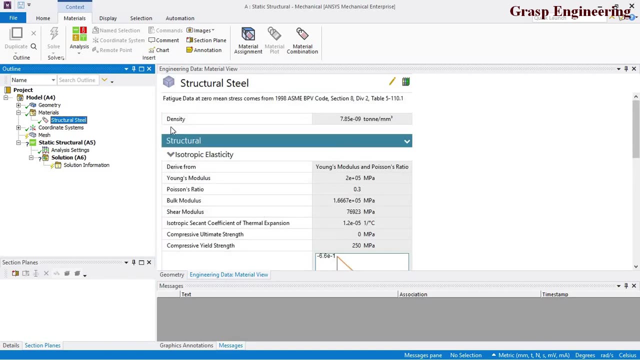 material by default. ANSYS will provide you a structural steel material. you will find that. what are the different material details as well as it will also give the stress life SN curve you can see like SN curve. so all the details for the respect to structural still are present over here. if you want, you can right-click and create mogą. 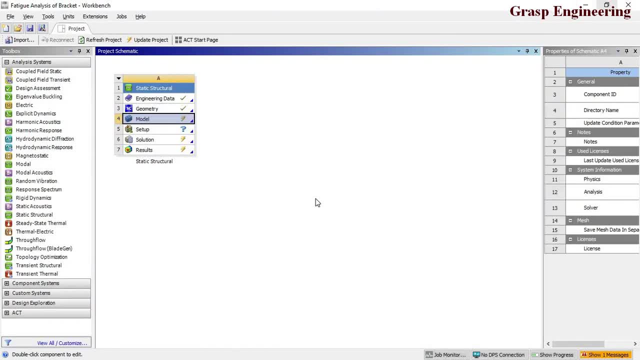 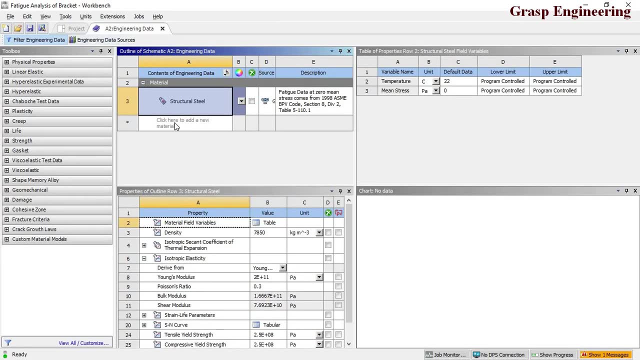 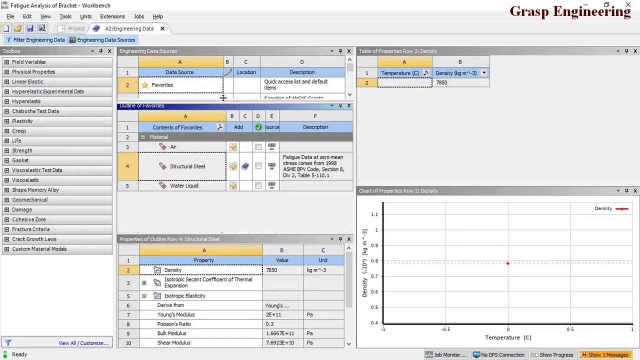 assigned. or you can create a new material also, or else you just go inside here, double-click under the structural engineering data sources and here you can refer a new material from engineering data source. okay, so now, if you see under the general materials, if you click on the 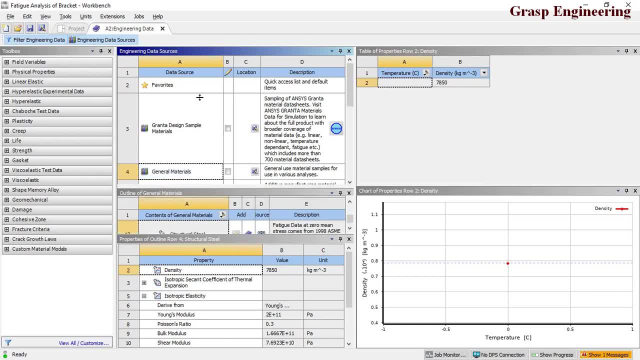 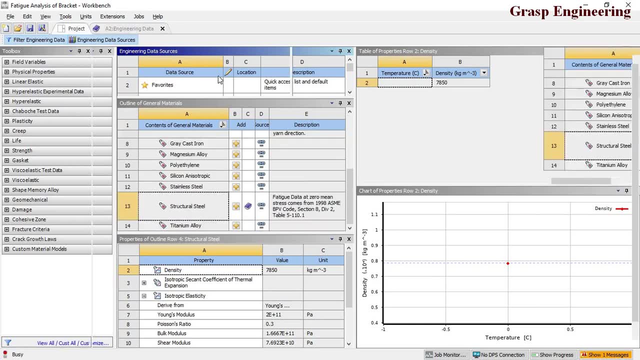 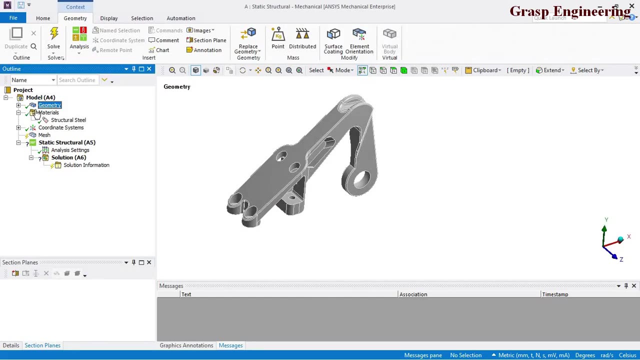 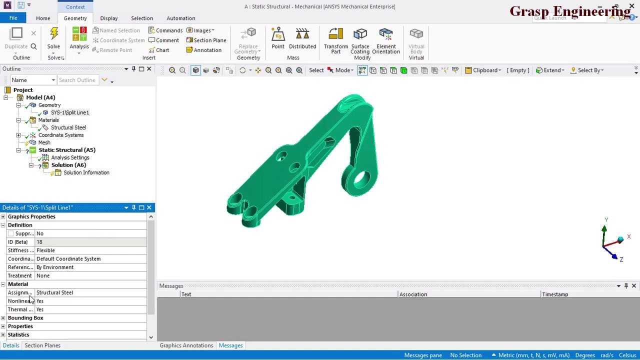 general materials. there are various materials um ansys library, so you can refer according to your product. okay, now let's go and in order to check the material whether it is assigned or not, you just need to click here, geometry, click here and under the details you will find that which material is assigned. so here you can see. 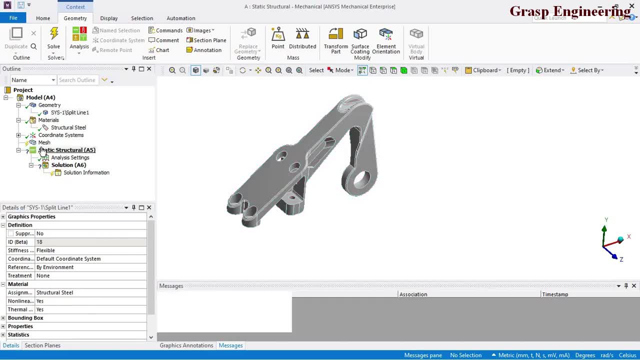 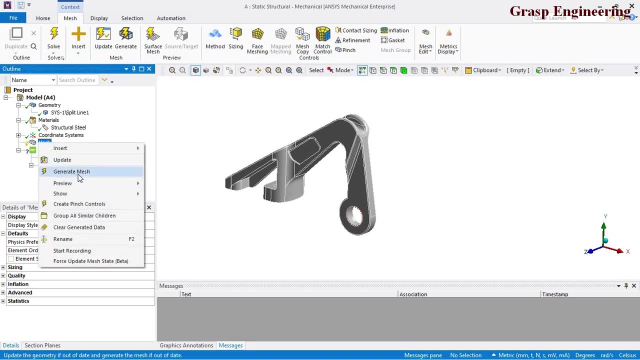 the structural steel material is assigned. now let's do the next part, that is, mesh generation. so at present we will not focus on the material- sorry, mesh generation part. so we will just directly use the global mesh sizing which is present under the mesh. and here you can see: 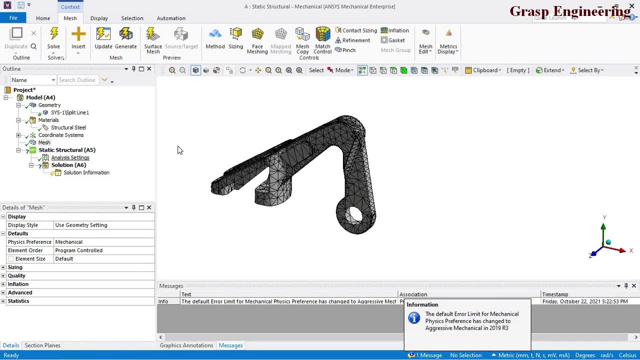 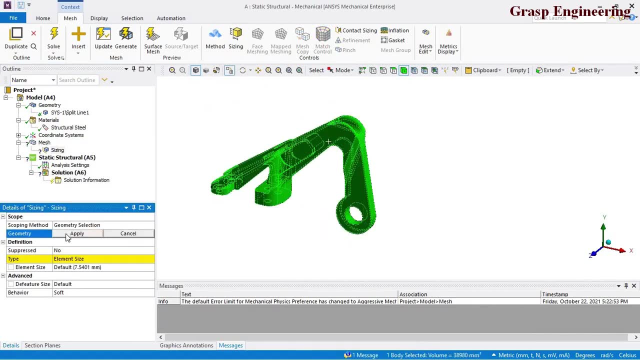 like global mesh, how it is going to be done, or in order to perform the local, right click insert and you can define your sizing. select the part here and here you can define your sizing, whatever the sizing you want. so let's make it three and generate the mesh. 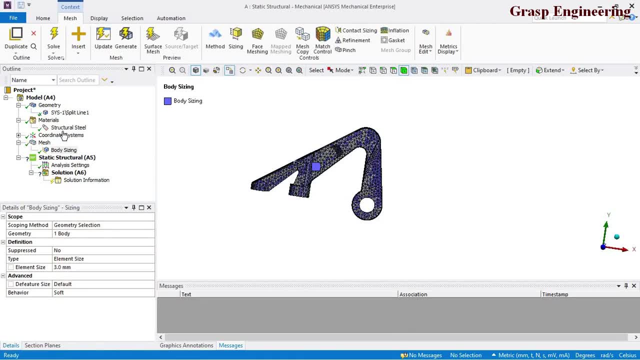 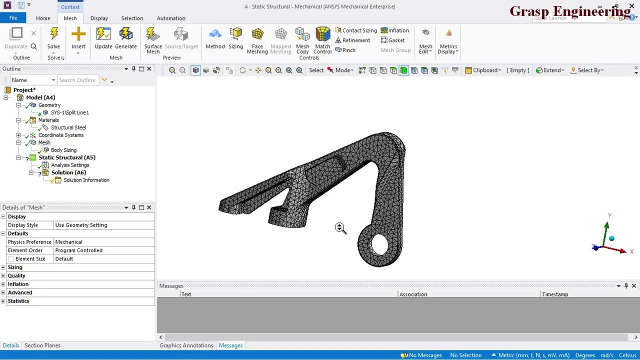 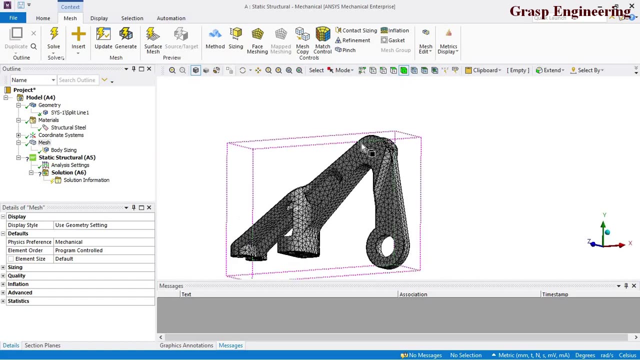 okay, make sure that while doing fatigue simulation, your mesh should be much finer. okay, because it should report the peak stresses, so we will just go with this moderate mesh. uh, you, when you will do simulation, at your end i will recommend you, or i will suggest you, to go with much finer mesh. 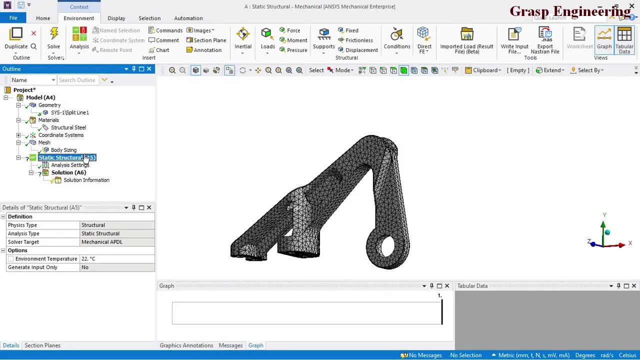 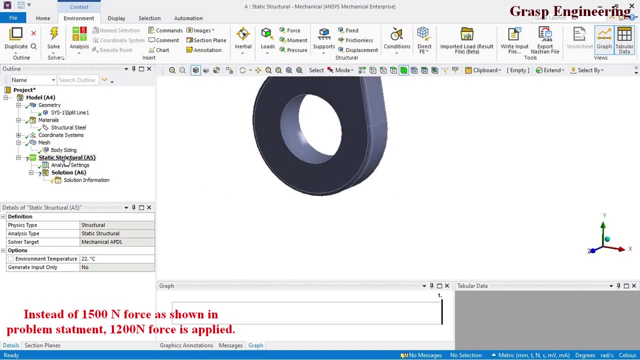 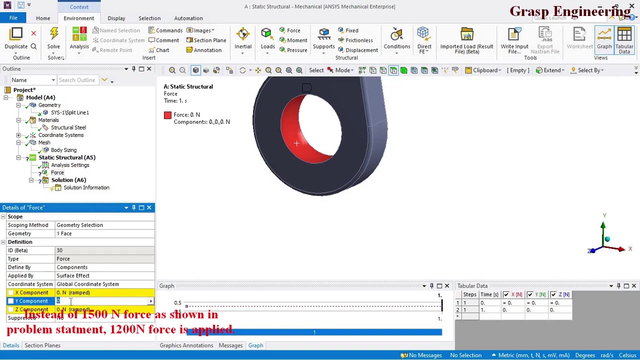 okay, now let's apply your loading and boundary condition. the very first we will apply our force, that is 1200. newton insert force. here you can see the force, select the face and here you can define the force in negative y. so for that refer component, let's go here minus 1200, okay. 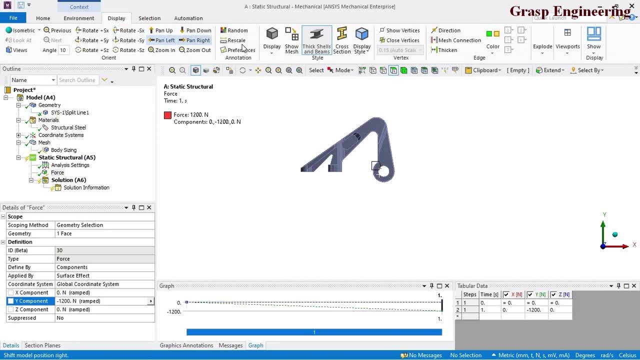 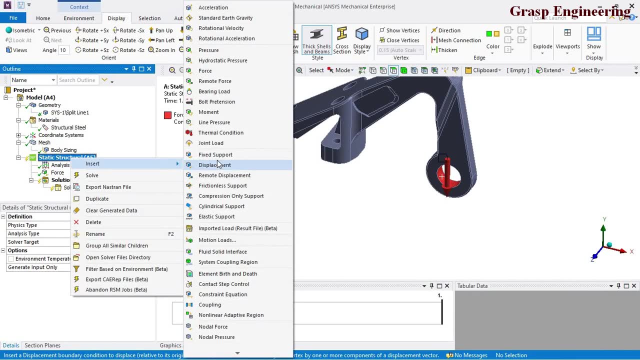 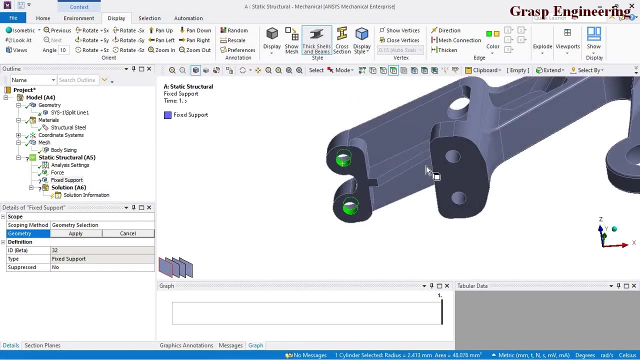 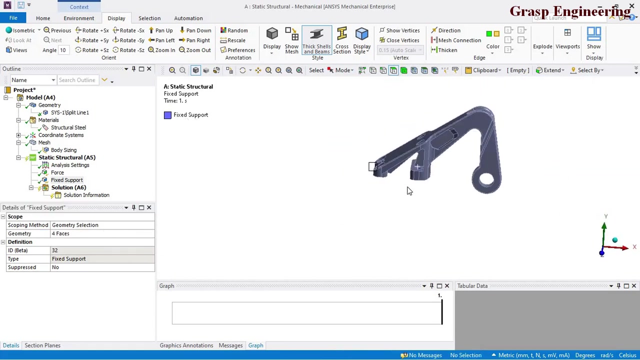 here we applied a force of 1200 newton. now the next case is to apply the boundary condition. so you just need to, as per the problem definition, let's select all the four faces, apply and lock all these degrees of freedom. so when you suppo keep fixed support, it means that 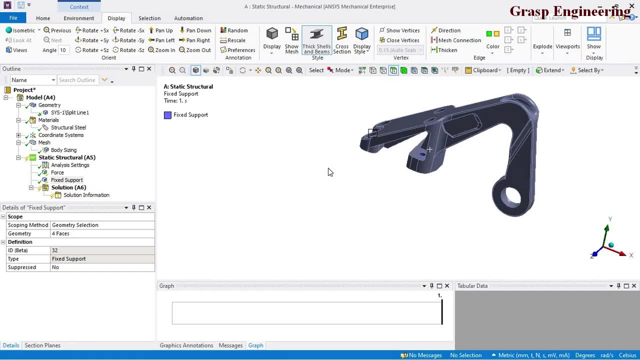 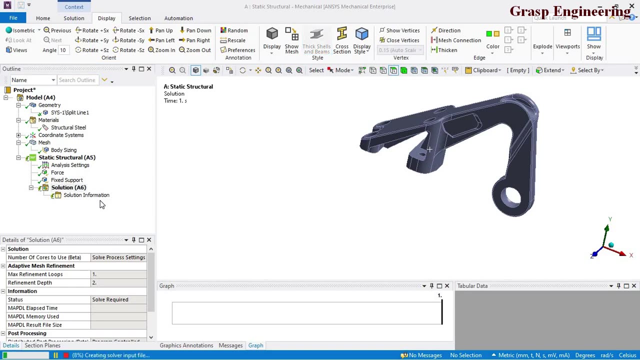 you are locking all degrees of freedom, so there is no and rotational movement. okay, now let's simulate this simulation. so right-click and solve. it will take some time to perform the simulation. so once your simulation is done, then you can land up or you can go with the fatigue. 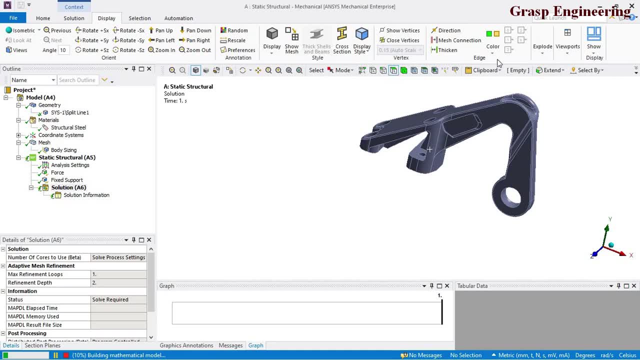 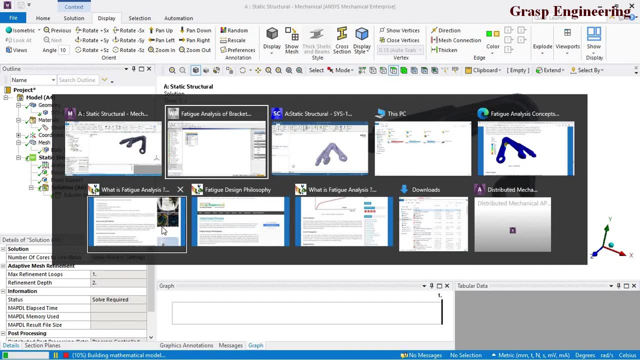 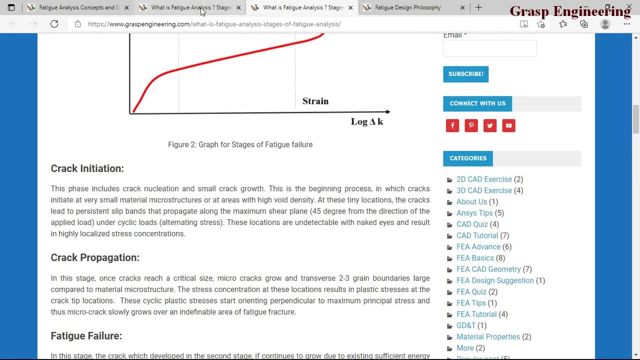 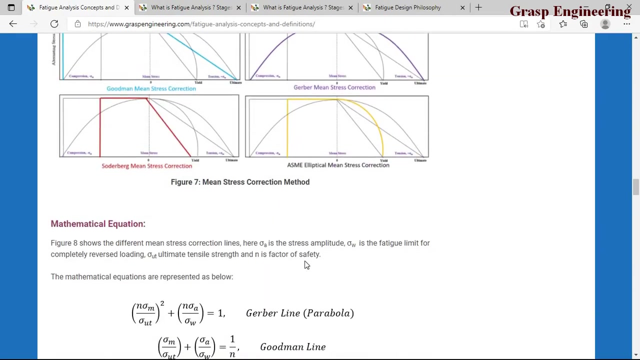 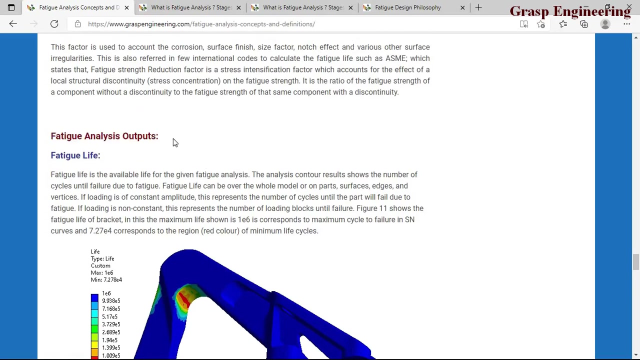 simulation. so which is basically the analytical, analytical part. so we have time, so I will just take you through further our blog post. so okay, so, while simulation is in progress, let's discuss few more terminologies, like: what are the fatigue analysis outputs which we need to look while doing the fatigue simulations? 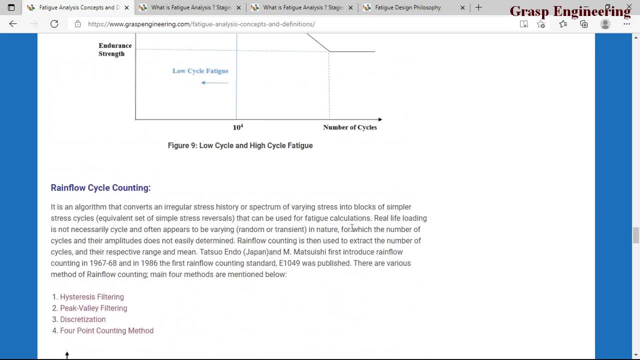 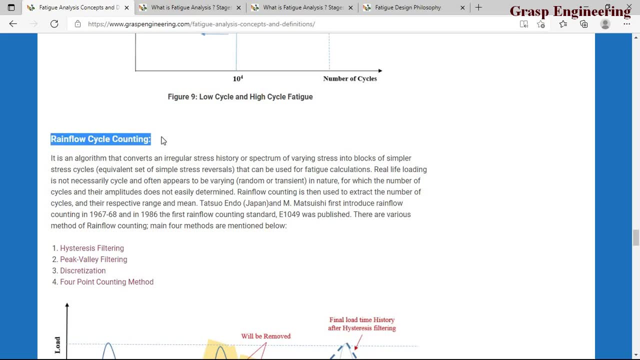 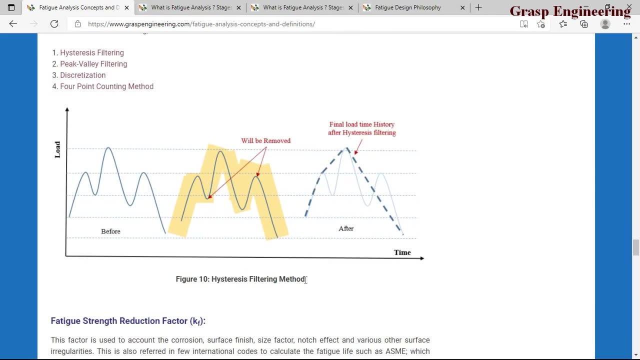 okay. so before that, let's discuss the reinforced cycle counting. so, as we know that one of the best or most preferable cycle counting method is a reinforced cycle counting, so if you see that there are different filtering methods, one of the method is like hysteresis filtering method. 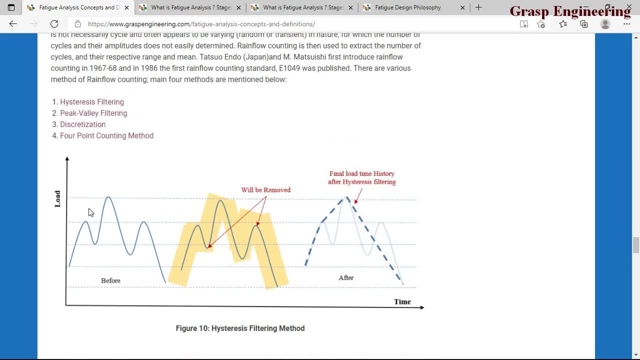 so in that method, what it does, just, for example, refer this graph. you will find that this is what the your complex cycle and if you see here what is your bottom point- this one, what is your maximum point- this one- and what is further your bottom point- this one- so if you see this last graph, 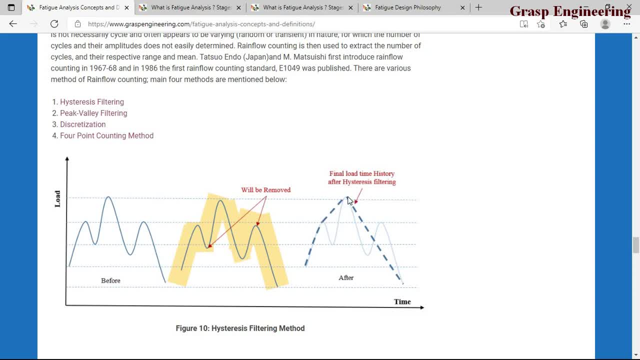 you will find that it will connect the extreme points within the cycles and it will eliminate the in between points. so you can see that these two points are eliminated and your one curve is created. so likewise it will does for all the remaining load cases. so what? in simple method, it simplifies your loading cycle. okay, from complex to 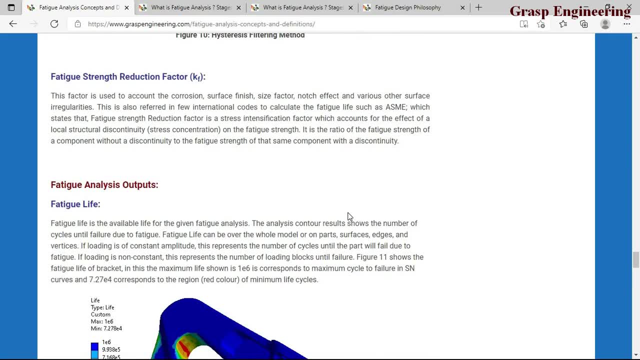 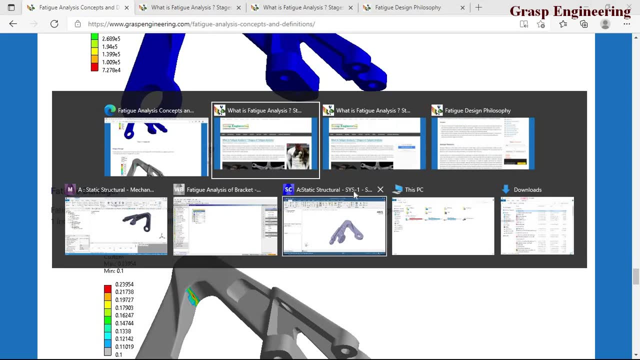 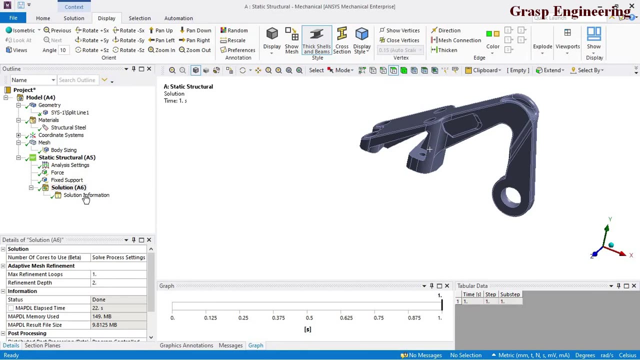 simple stress cycle. now let's talk about the fatigue analysis output. so let's first check the simulation is done or not. okay, so we will do later on. now, if you see our simulation is performed, uh, let's check the deformation and stress cycles. so i'm just doing the simulation live in front of you, so don't think that it is though we are. 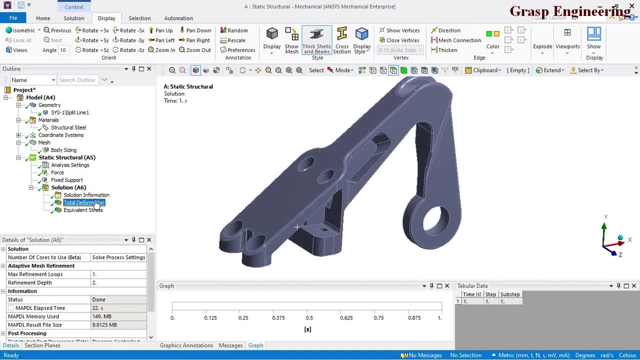 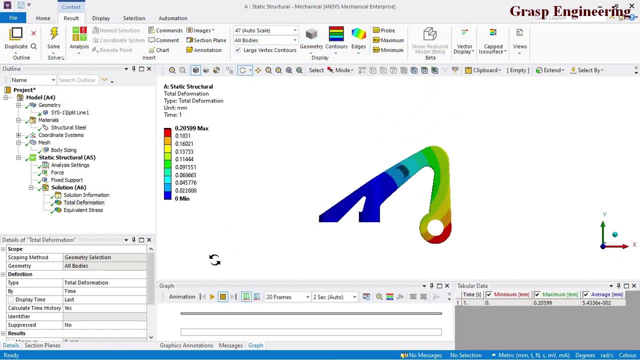 we did the recording, but the simulation is live now. if you see that, uh, the deformation, let's check through the animation. okay, so it should behave like that only because we are applying the downward load. so deformation is quite uh low, like 0.2 mm. let's check the stress cycle. 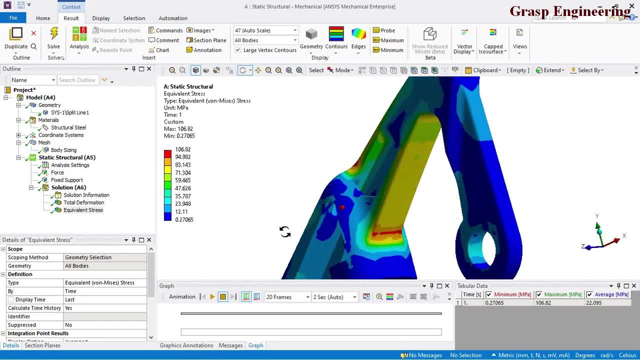 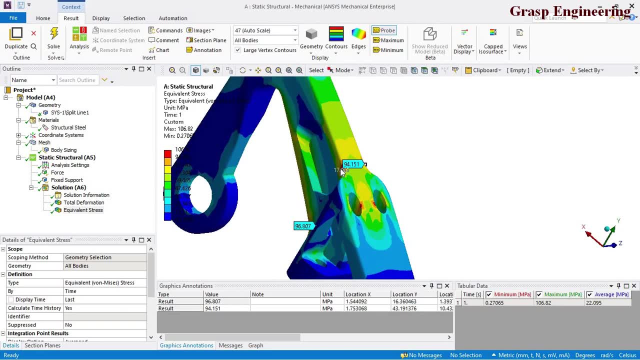 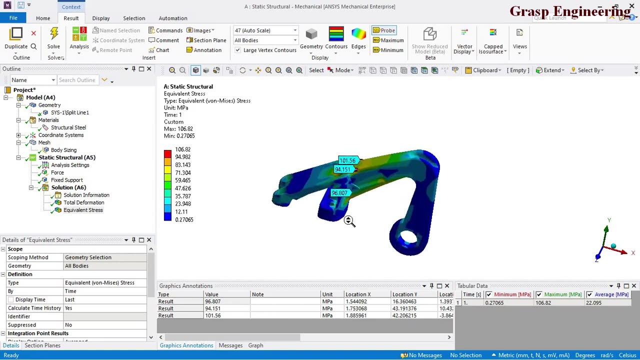 uh, stresses. so if you see here the maximum stresses we observe at these points, here as well as at this location. so these are the critical locations where you will find the alternating equivalent stresses. okay, always remember where you will find the highest stresses in static simulation. at the same time, you will find the higher stresses in static simulation. 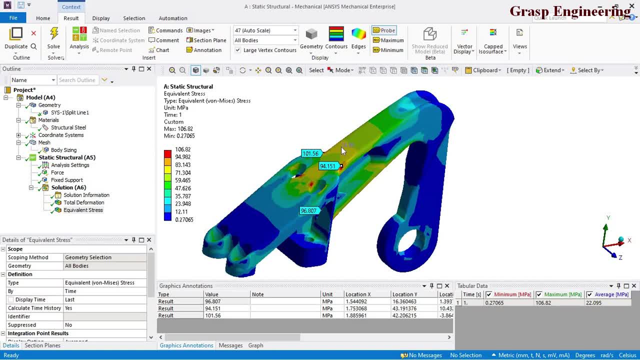 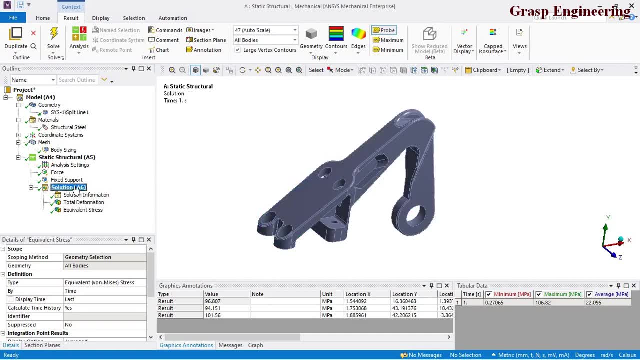 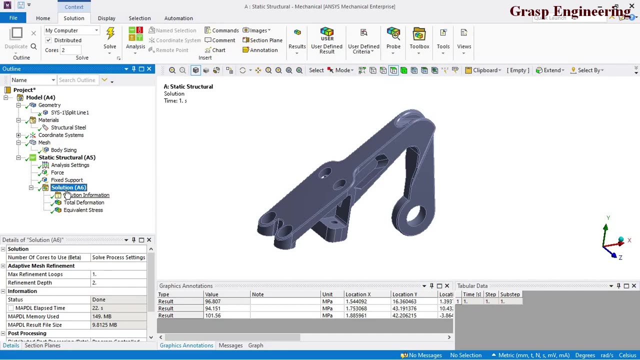 point. you will find the alternating equivalent stress in the fatigue simulations if you have a constant loading, now let's do this. our fatigue simulation, which is was the area of interest of our present video. so in order to perform the fatigue simulation, you just need to right click. 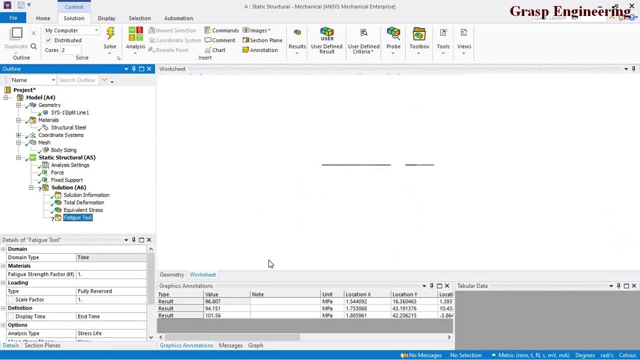 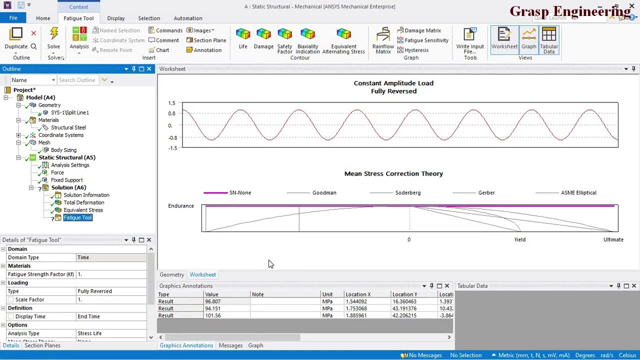 insert and here you can find that fatigue tool. so when we talk about fatigue analysis you might confuse that we need to do a separate simulation. you can do the separate simulation. there are different softwares are available in the market, just as at present your ansys even. 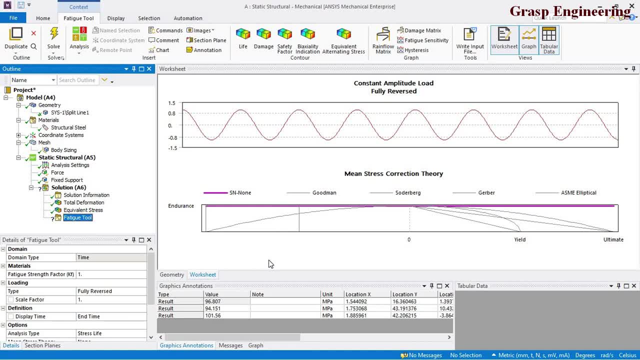 there is one more software called encode which is widely used to perform the fatigue simulation for a complex loading. there are few other simulations like abacus, solid, solid work, but there also a simplified fatigue simulation, nastan pad. so these other software are available in the market. are there you where you will find the fatigue simulation? even there are few tools where you 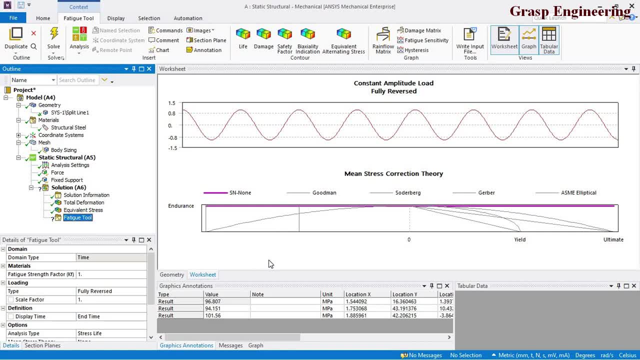 can, which are actually form just to perform the fatigue simulation, just like encode. present simulation is basically based on your this static analysis result. so the fatigue simulation is nothing but your post processing part. so, based on your SN curve for the respective material and based on your, your loading outputs, 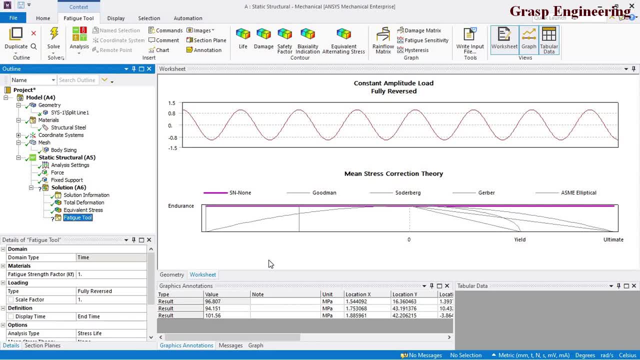 like peak and valley condition. it generates the life cycle and other fatigue analysis output. okay, there is no separate simulation. we are just doing. we are just referring the static analysis result and, based on your material inputs and loads inputs, we are just calculating the fatigue analysis output. so when you import the fatigue, you will find that, as we discussed at the beginning of video, there are 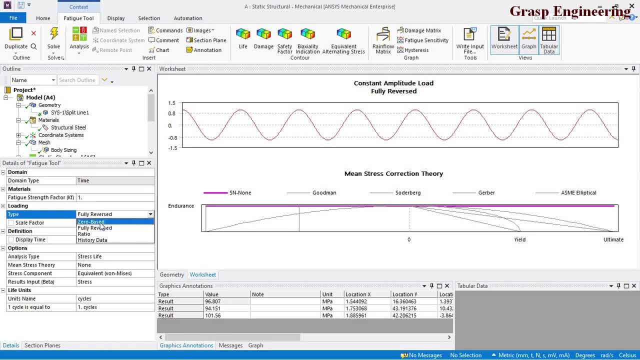 different load types. so you can see the load types are different. so you can see the load types are: changca área MUSIC. so when we talk about zero base, so you can see it is wearing from 0 to 1. like that, when we talk about fully reverse, so minus 1, 2 plus 1, and we talk about the ratio, you 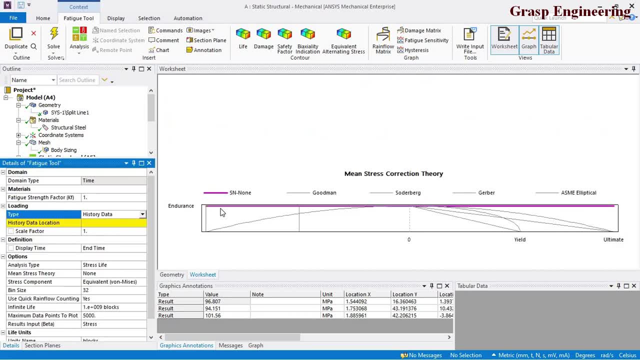 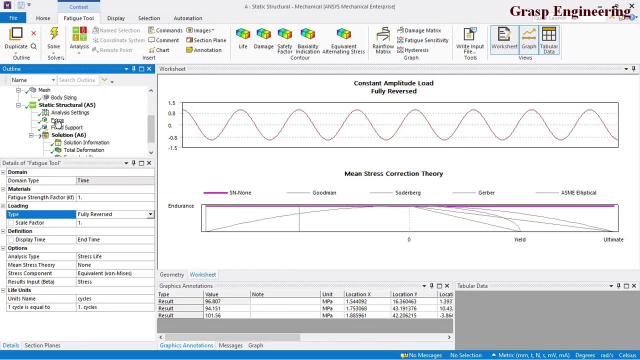 can see, right, and you can see the history data. so it is basically for when you have a variable amplitude, you just define the path and you can read that file. okay, at present, let's consider the fully坐 a cycle. okay, so what we are doing? we are assuming that this respective load is varying from positive. 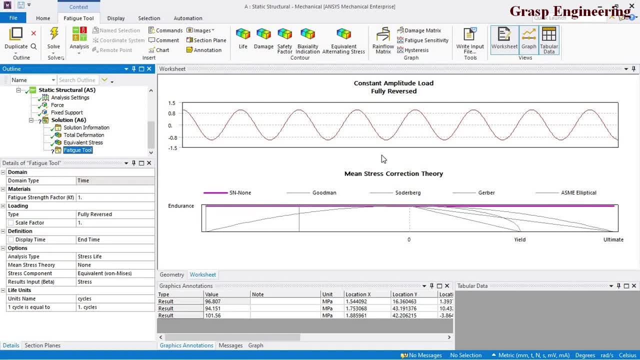 to negative. you know, you can see like this. and now let's check the analysis type. so, as i discussed earlier, there are two approaches, main two approaches, like stress life and strain life. so let's simulate the simulation with strain life and, as we discussed earlier, there are different. 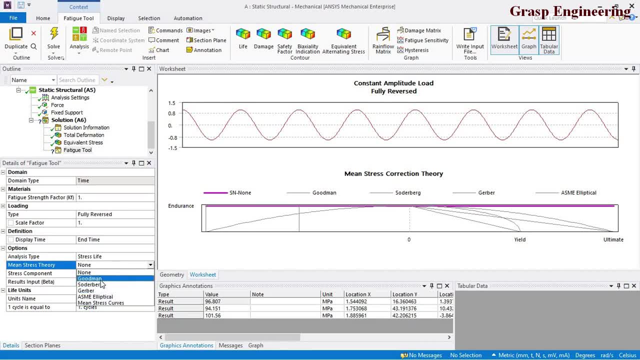 theories of mean stress corrections. so let's consider the goodman stress theory and let's consider the equivalent stress to calculate the fatigue life. okay, and here the results. what results you want? either a strain or stress. so let's check these stresses, okay, and inside that, once you define your loading condition for a fatigue, right click insert and you will find: 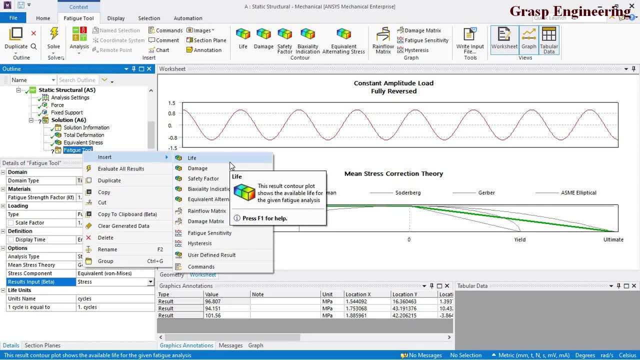 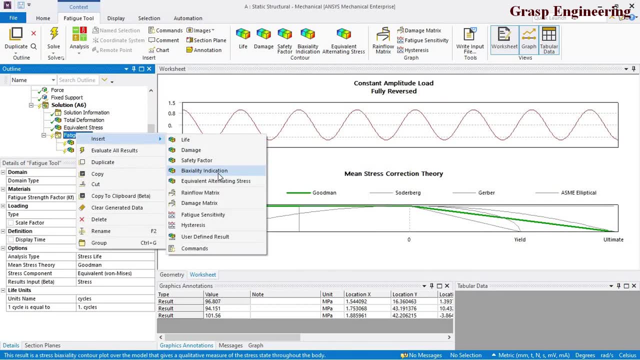 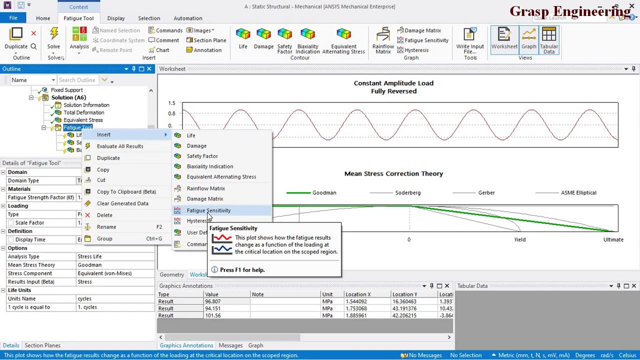 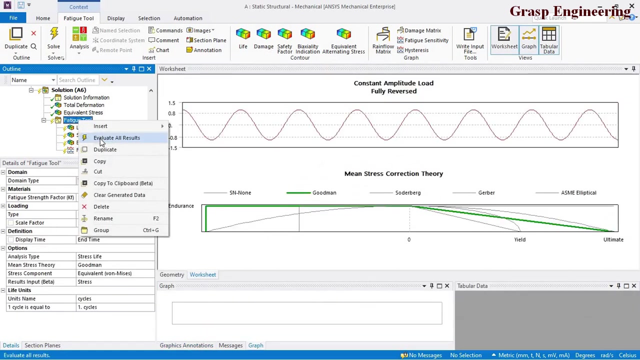 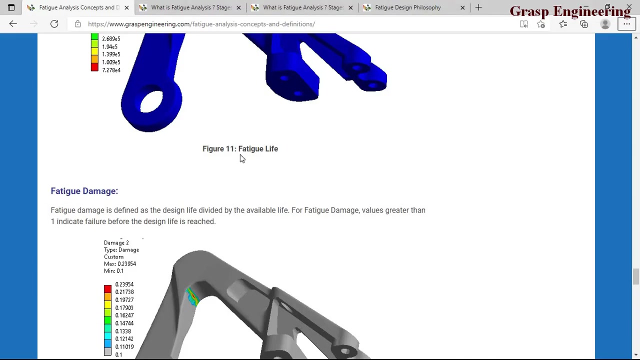 there are different fatigue outputs, just like your life, uh, just like your safety factor, just like your binding by excel indication. and let's talk about the fatigue sensitivity. okay, so, before discussing all this parameter, let's evaluate this reason. what we will do: we will go to our blog post and there i will just explain you. what are these different terms? are there? 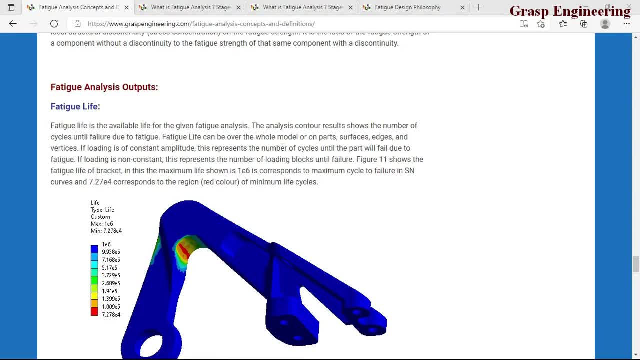 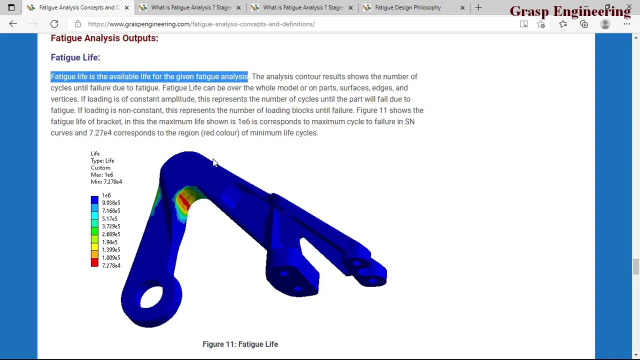 so now let's discuss about the fatigue analysis output. the very first outputs we are interested for a fatigue simulation is fatigue life. so when we talk about fatigue life, it is nothing but the available life for a given fatigue cycle. so if you see this respective counter plot, you will find: 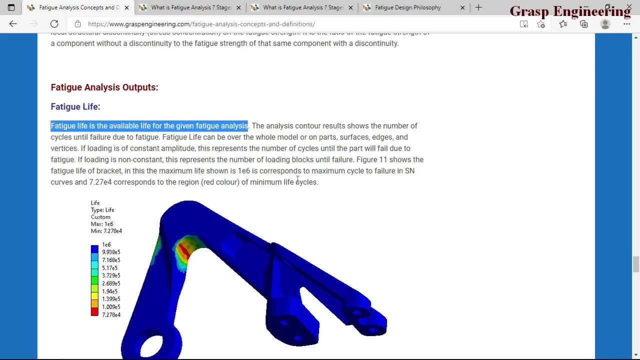 that the maximum numbers belongs to the cycle. you can see here, like in this figure 11 shows that the fatigue life of bracket, the maximum life 1 raise to 6, is corresponding to the maximum cycle to failure in a sn curve. so when you refer any sn curve you will find that the different life cycles the maximum. 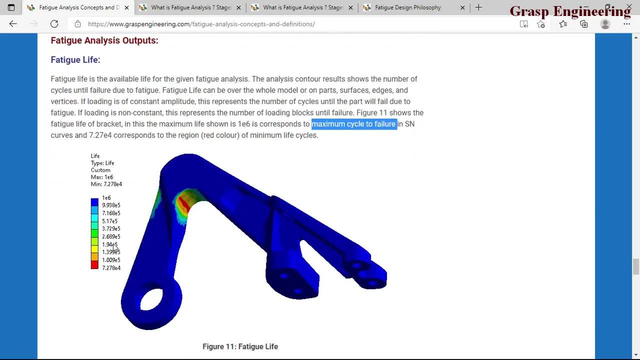 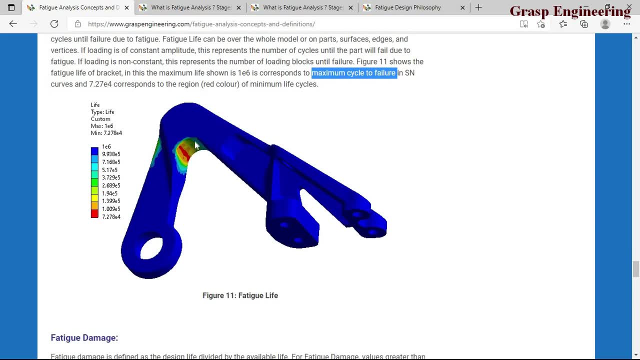 cycle to failure is nothing but your this maximum cycle, okay, and this known is no more than 1 severe minimum cycle- corresponds to the minimum life cycle of this respective component. when you refer the color, this respect to legend through the color code, you can easily identify. if you probe your cursor here at this respect to, you will find. 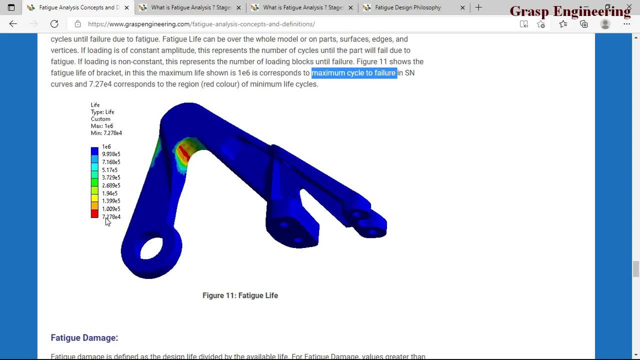 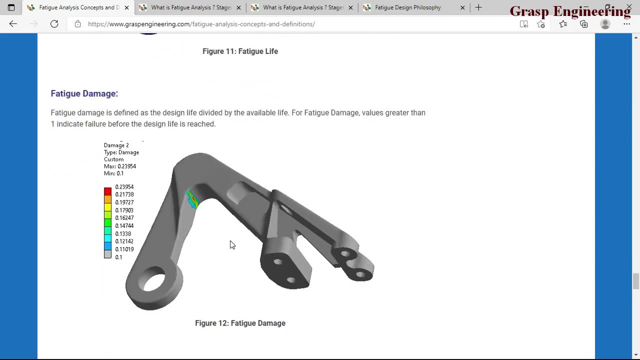 this life cycle is in between the 1 e raised to 5 to 7.27 e raised to 4. okay, so minimum a life cycle this respective component will withstand is 7.27 e raised to 4. now the next important factor of output of fatigue. 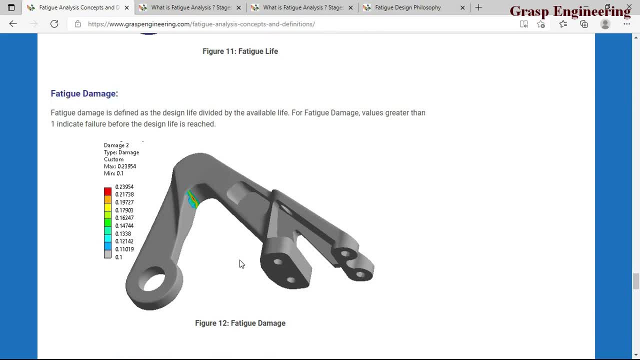 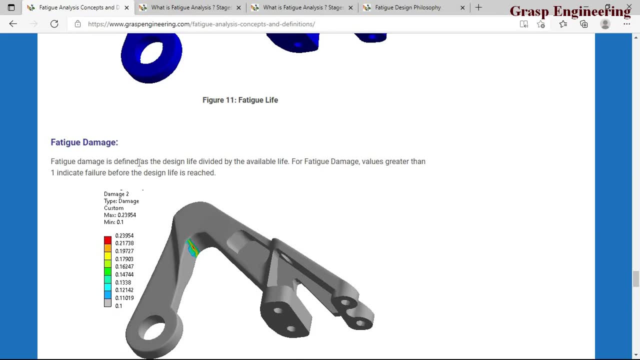 simulation is fatigue damage. so when we talk about fatigue damage, it is also as same, as it will also display in the similar fashion, but here the fatigue damage is nothing but the ratio of design life to the available life. okay, so basically whatever. though, when you refer any product, you should. 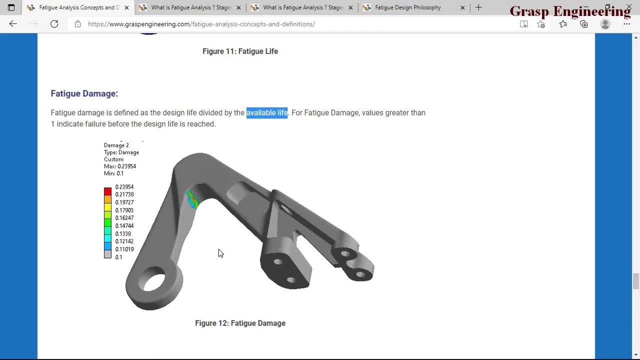 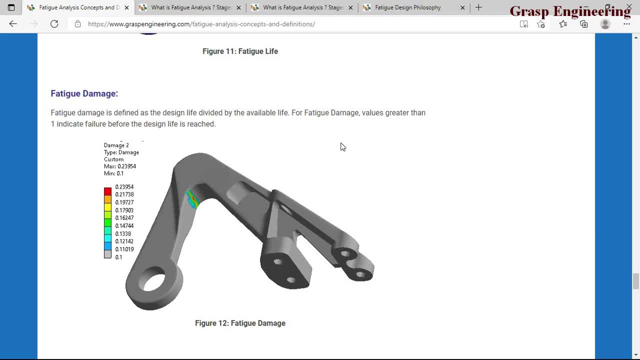 life to all is nothing but your fatigue damage. so for fatigue damage, values greater than one indicates the failure. so always remember fatigue damage should be below one. okay, when we we say that your fatigue damage is below one, it means that your component is safe. when we say that our 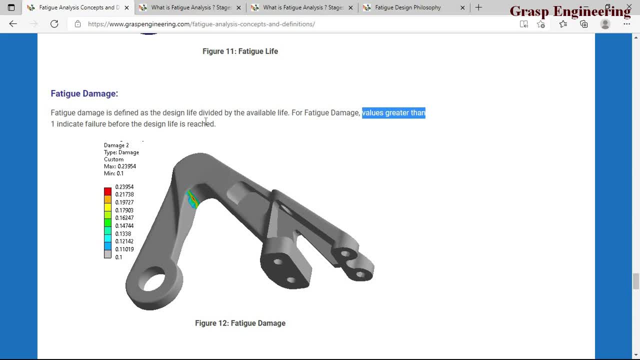 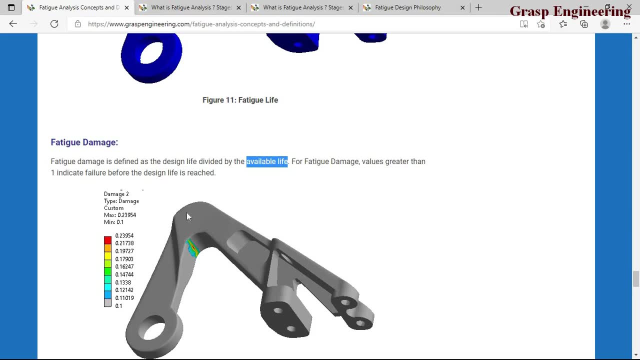 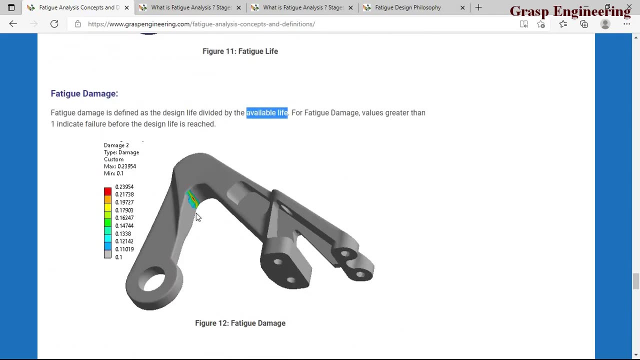 fatigue damage is greater than one. it means that whatever the life which you got is not exceeding the design line. okay in simple, so always choose the respective probe values. uh, the, here you can easily probe the values like if you want to see. here your fatigue damage is. 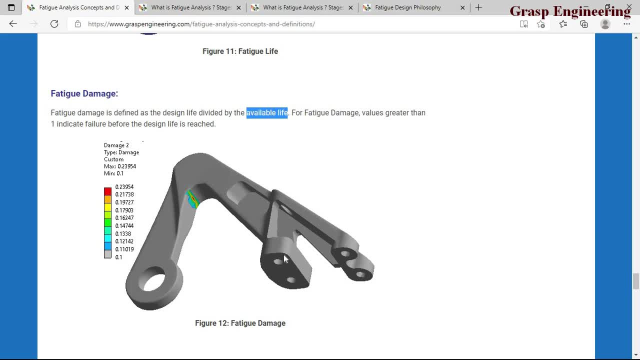 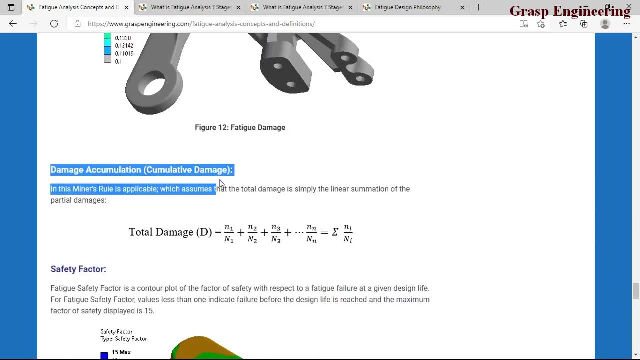 0.23. if you probe here, your fatigue damage is 0.1. okay, now let's. uh, the important terminology is safety factor. this damage accumulation is nothing, but it is just the sum of your fatigue damage for the respective number of cycles. when you have different number of cycles, you can easily simulate. 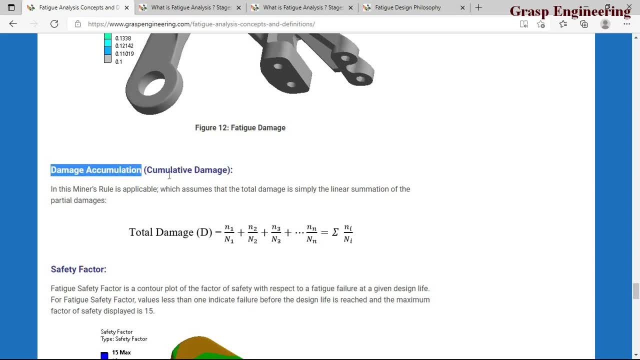 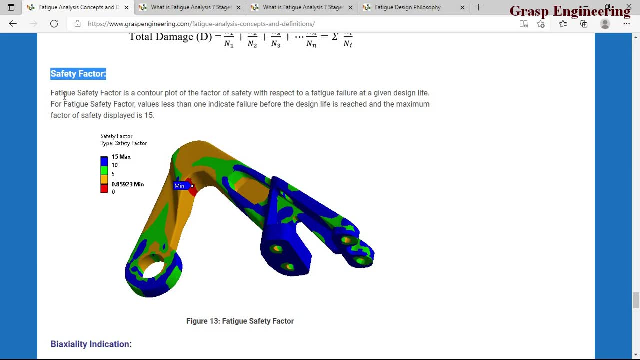 that and cumulative thing is nothing but your cumulative fatigue damage. now let's discuss, uh, one more important parameter, that is safety factor. so the fatigue safety factor is a counter plot of factor of safety with respect to the fatigue failure at a given design life. so basically, it is nothing but the factor of safety. 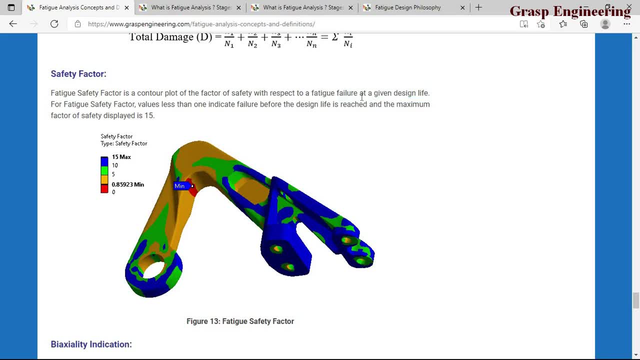 with respect to your fatigue. failure for a given design life. okay, now, when we talk about the value less than one, it indicates the failure before the design life is reached and the maximum factor of safety displayed is 15- 15.. so, if you see this, uh, religion, you will. 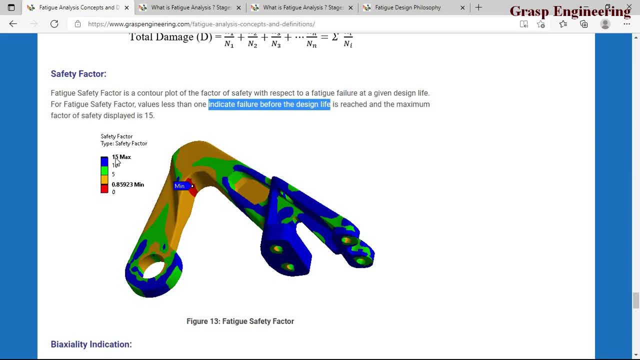 find that the maximum value which is displayed is 15 and the minimum is varying from 0 to 1.. so it says that when the values indicates less than 1, in that case we can say that it will going to fail before it will reach its design length. okay, so for that uh indication, it is. 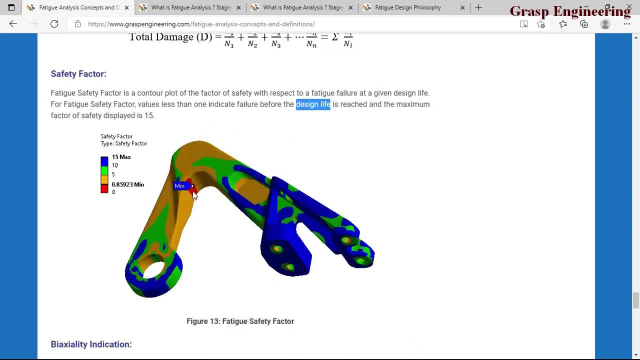 cool to see the safety factor. so if you see here this color code reason which represent 0.85, 9, it is nothing but the critical reason, or you can say that the failure will going to happen at this respective location when you apply the further fatigue load before reaching is design. 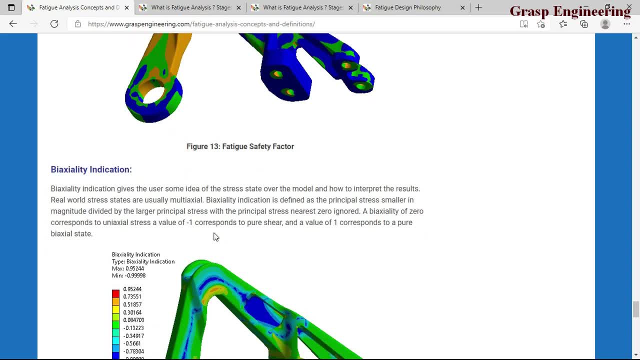 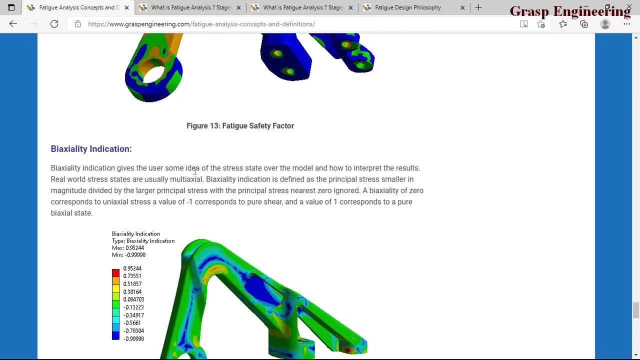 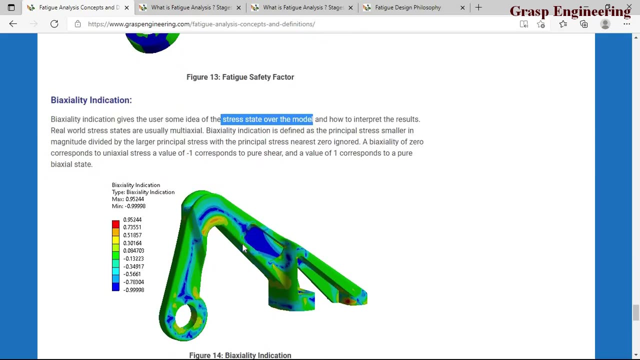 line. now let's talk about one more important parameter, that is, biaxiality indications. so when we talk about biocically indication, it gives the user some idea of a straight or the model ok, so basically it shows this state of the stress. so when we say that, if you see, refer this respect. 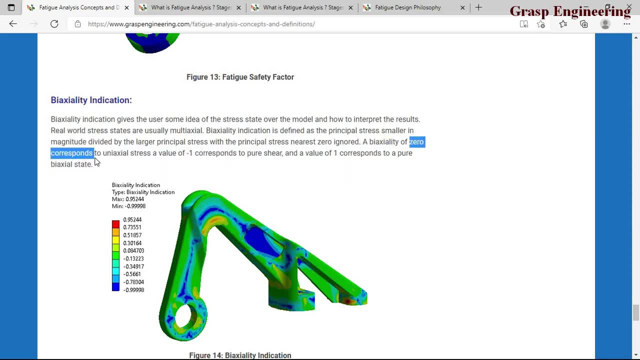 to legend. when we say that the biaxiality is equal to 0, it corresponds. 0 means somewhere. here it corresponds to the uniaxial stress value. ok, so if you see here this color code, here you will have the, the uniaxial stresses. When you will say that your biaxial indication is 1, it corresponds to the. 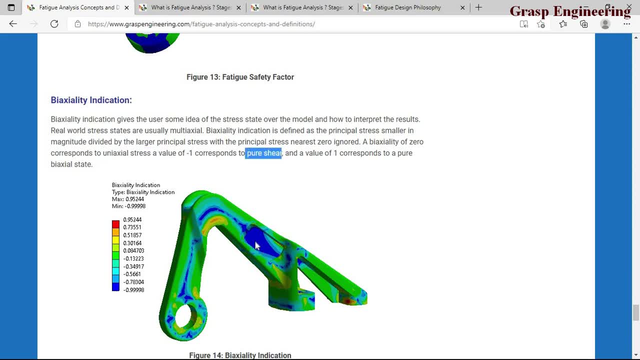 pure shear condition. So minus 1 somewhere here here you can see it states the pure shear state. Now when we say the positive 1 value, it is nothing but the pure biaxial state. So positive 1 means the maximum values. I think somewhere here you can see, inside this location. So 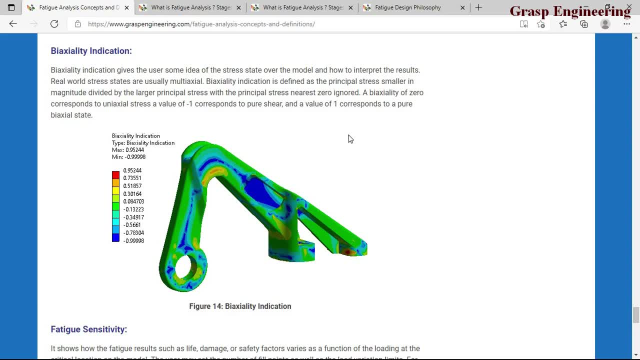 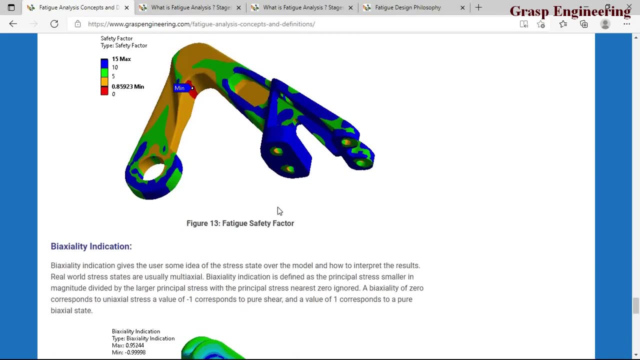 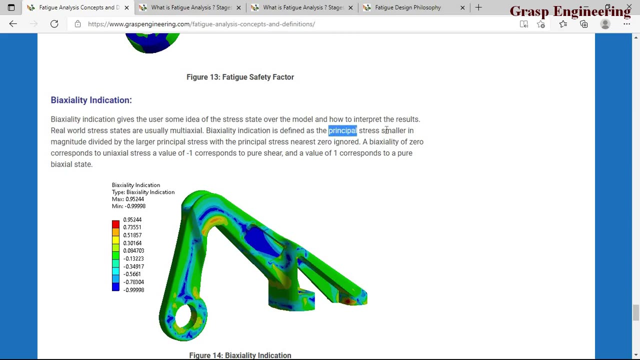 this is nothing but your pure biaxial state. So it might confuse you while referring this, but when you do the number of simulation then you will come to know that how to interpret this respect to output. So it is nothing but the biaxial indication is the ratio of. you can say 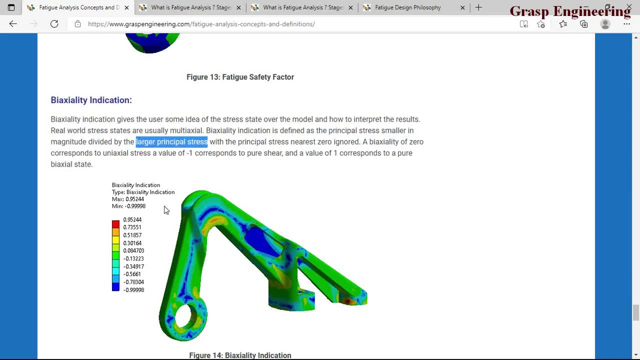 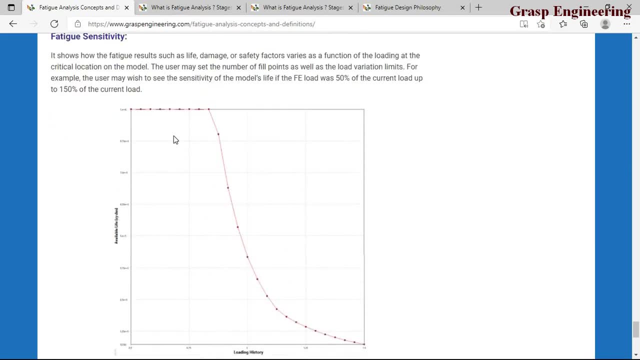 maximum principal stress to the larger principal stress. Now, the next important parameter is like fatigue sensitivity. So let us what does it shows that. Let us take an example of like you are applying a force of 1200 Newton. Now, if you want to see, 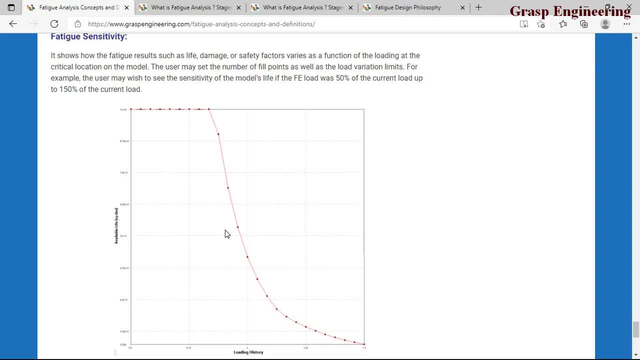 the results for like 200 percent load factor, like instead of 1200,. you want to see the result for 2400.. So whether you need to do the simulation. Similarly, if you want to apply a 50 percent load like instead of 1200 Newton, if you want to apply a 1600 Newton, 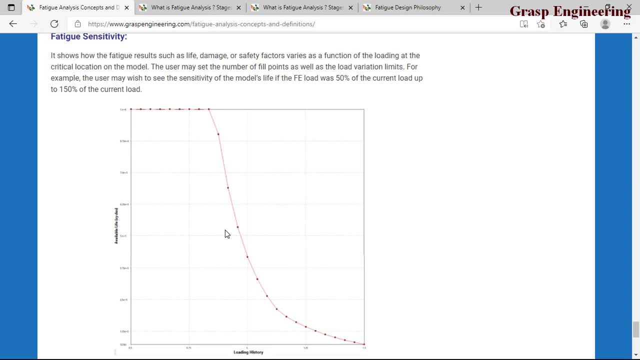 whether you want to do a further simulation. In that case, you can say no if you referring to this respect to fatigue sensitivity chart. Okay, So what it does? it basically varies your load value from minus 15 percent to the 150 percent, So you can even put that value like 10 percent. 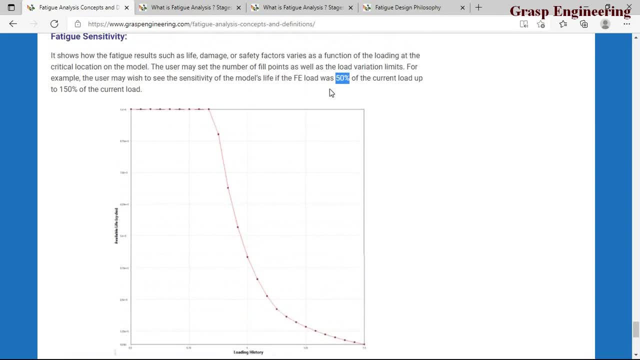 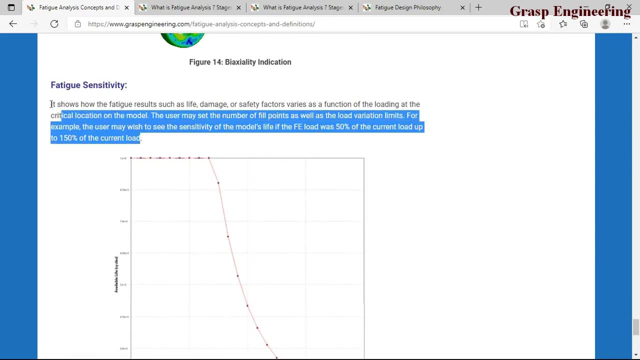 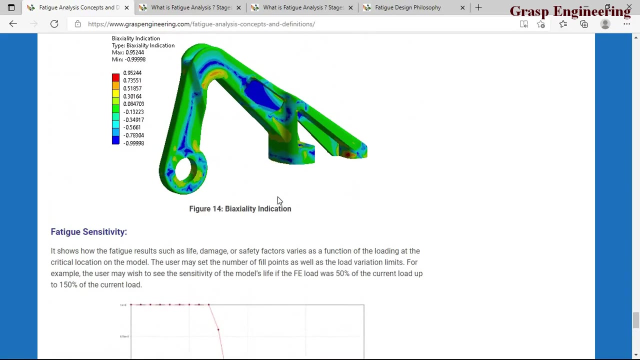 2 percent. So based on that respect to load minimum to maximum, you can easily interpret the design life. Okay, That is what this fatigue sensitivity shows, What we can do. now we can go to our answers and there we can see how to see this. 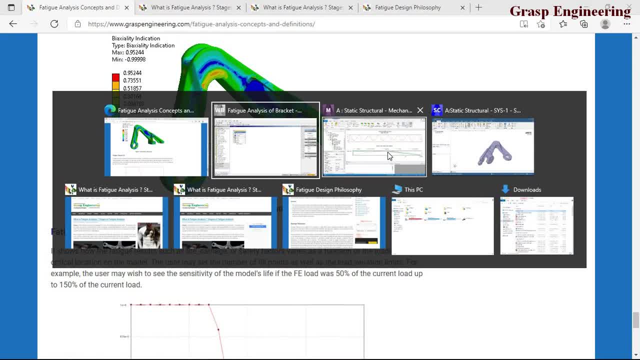 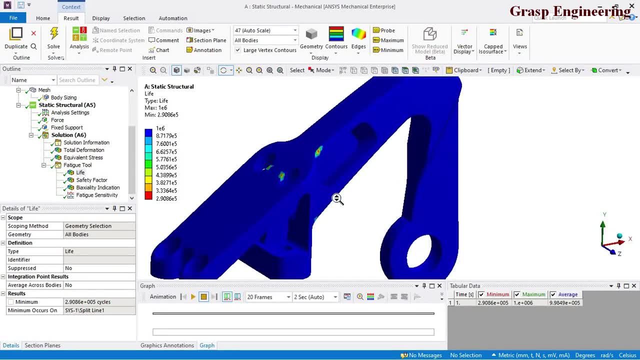 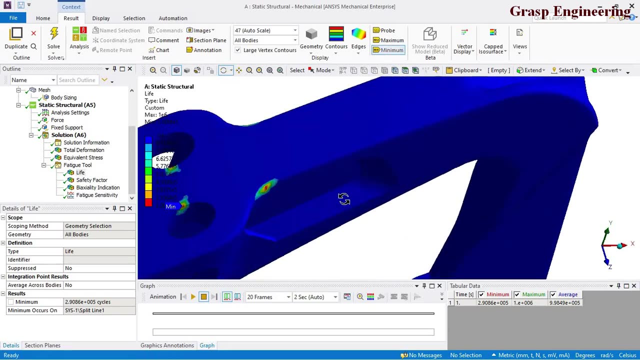 result Now, if you see that we had received our outputs. The first one is like fatigue life. So let us see what is the fatigue life? Now you can see like here: these are the critical parts. You can probe right, Even you can probe over here. 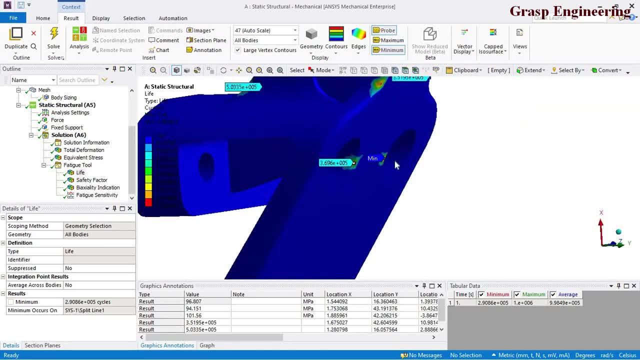 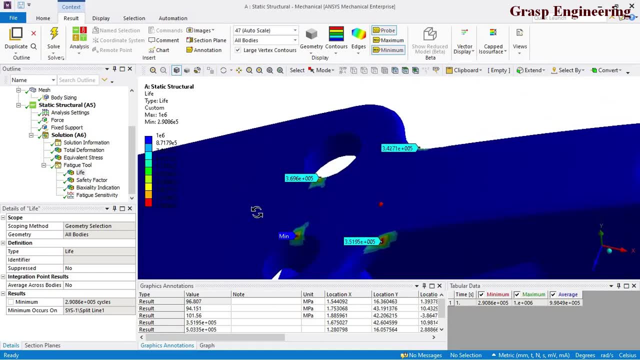 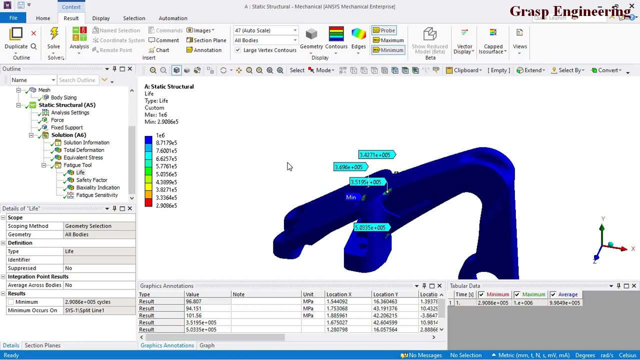 You can probe this respect to region. This might go when you do the further fine mesh. So that is why mesh is very important in this case. So you can see here the minimum life is 2.9 p raise to 5.. Okay, 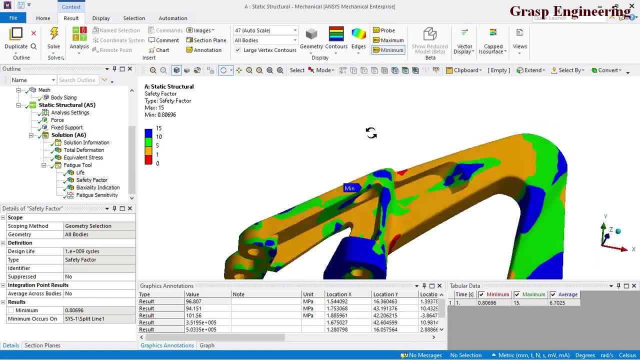 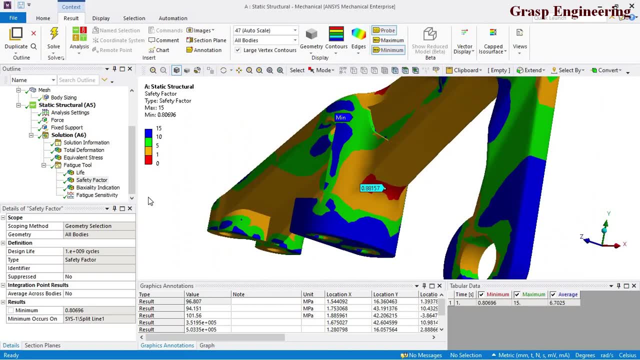 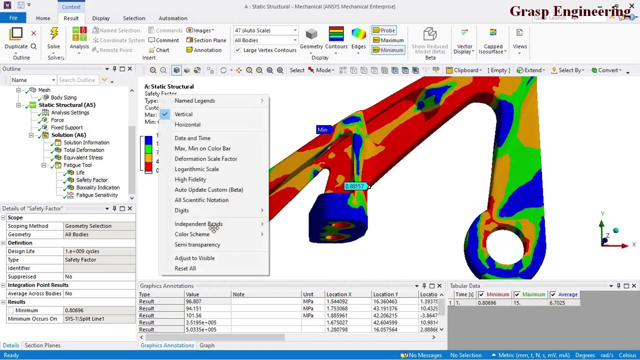 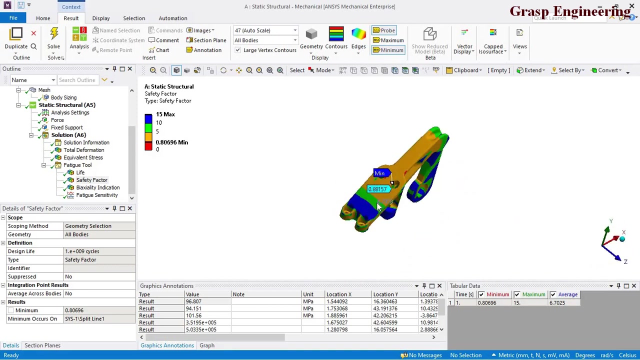 The another parameter is like safety factor. So, as we discussed, safety factor, you just need to check, so not single factor. you just need to check here because you, as you, as this only factor is just only factor, you just need to check whether it is So this one, this is the critical reason which So. 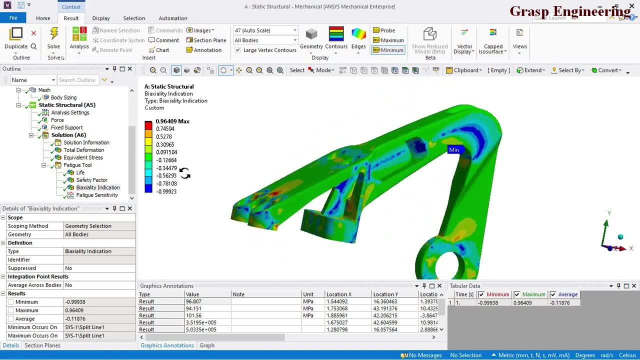 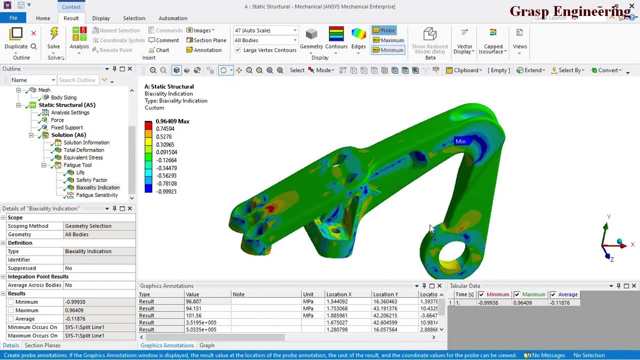 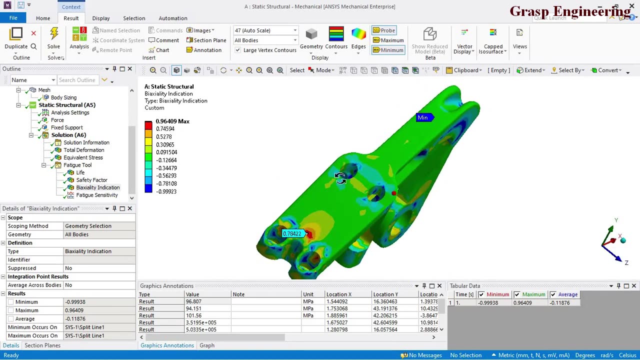 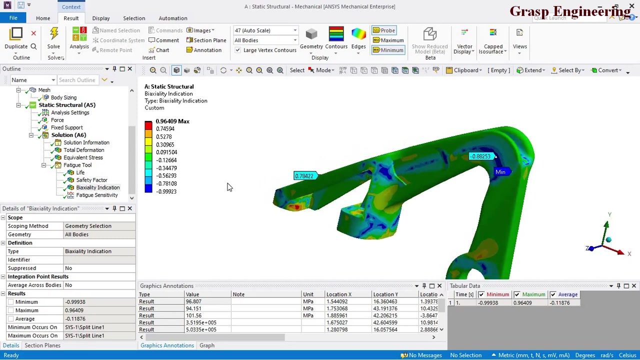 we can say that successfully. Okay, Now we can see 0.96. so when we say this value somewhere here it's straight, your pure by axial state minus one is here your shear. and when we say one or here, somewhere middle, it is your uniaxial state. now let's check the another important 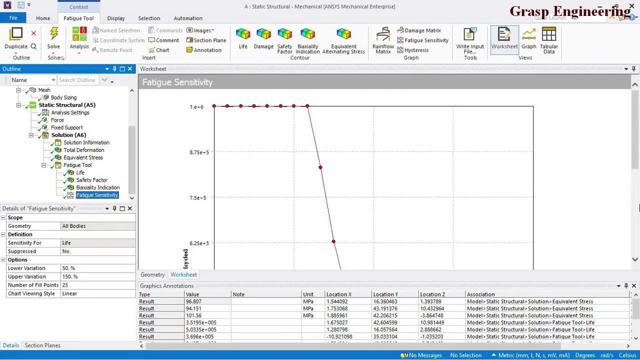 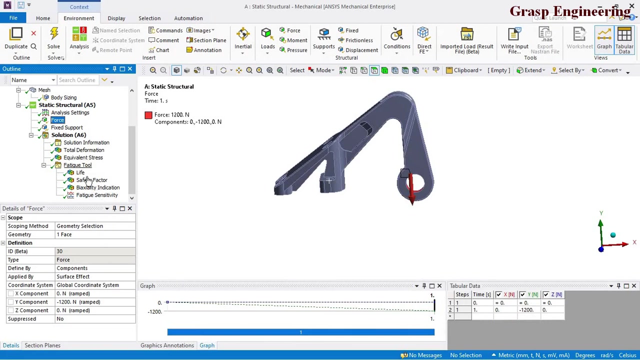 parameter, that is fatigue sensitivity. so as we applied here, like 50% to 150%, you can even vary that. also, let's make it 200% and evaluate the results. so when we say the, now let's talk about our force value, that is 1200 Newton, and for that 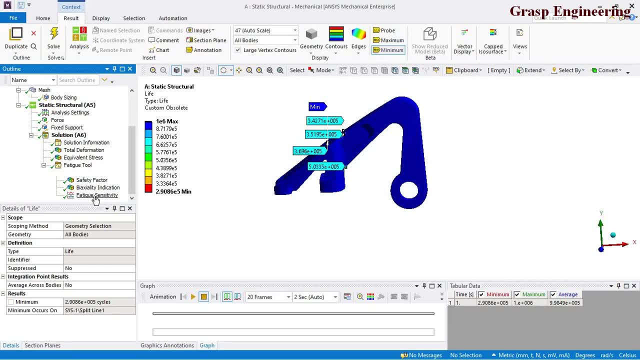 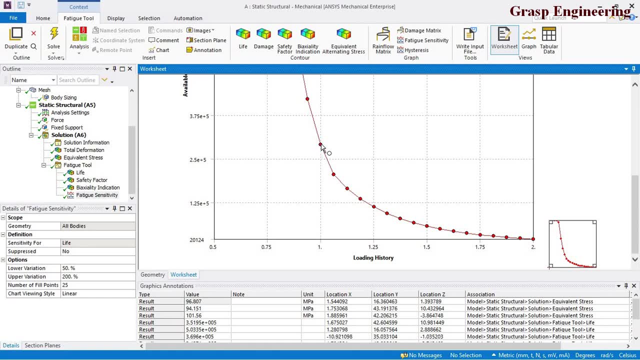 we receive the design life is like here: 2.9. so let's check here here, right, so this is what our one load, the maximum load, and for that respect to 2.9, we saw a raise to 5. now suppose if you increase the load further, like if you goes on. 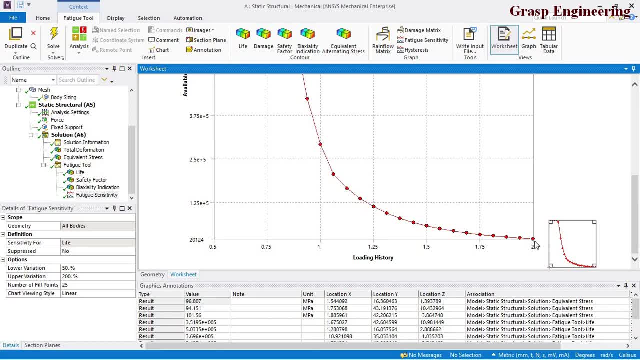 increasing load like two times, your fatigue life will drastically reduce to 20 000. suppose if you increase by 1.5 times, then your fatigue life will be in between, like here, 40 to 30 000. now suppose if you further reduce your load from 1 to instead of 0.75. so let's go up. 0.75 means here: 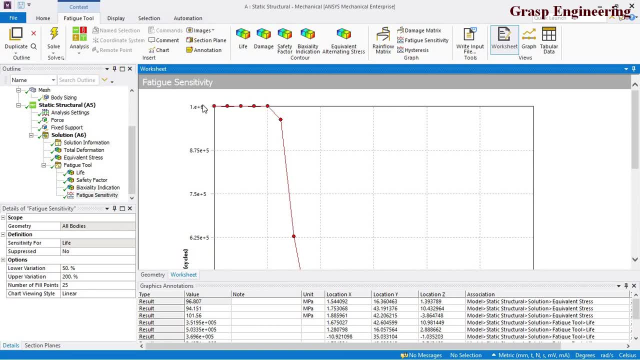 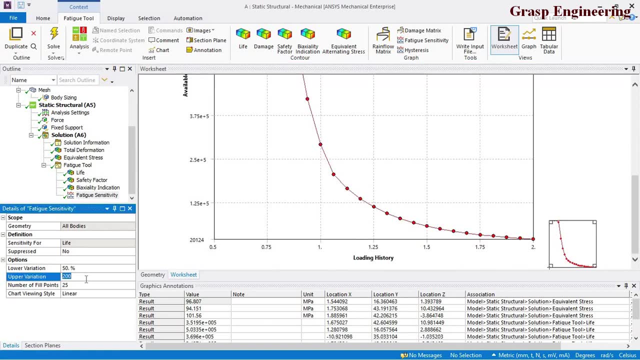 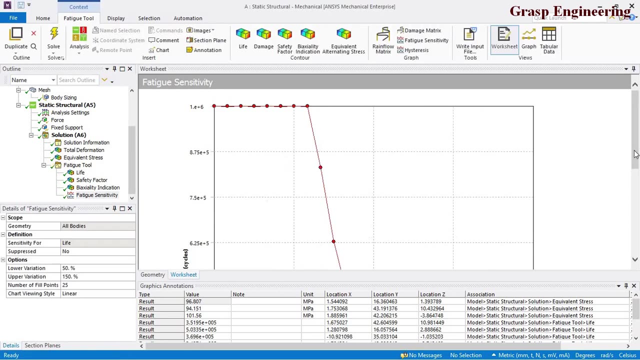 so your fatigue life will increase to 1.10, raise to 6. okay, that is what the advantage of fatigue sensitivity? so you can easily vary these values and you can check the respective graph instead of performing the simulation. so if you check here for 1.5, it is 56. 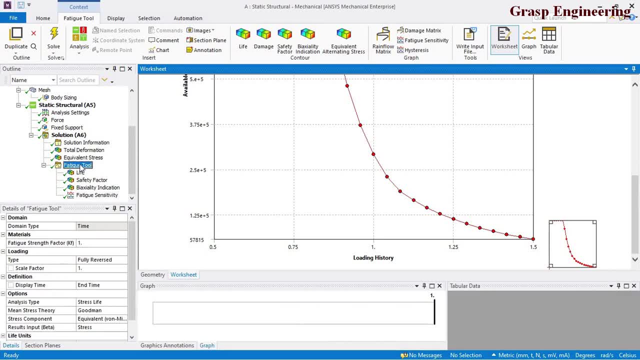 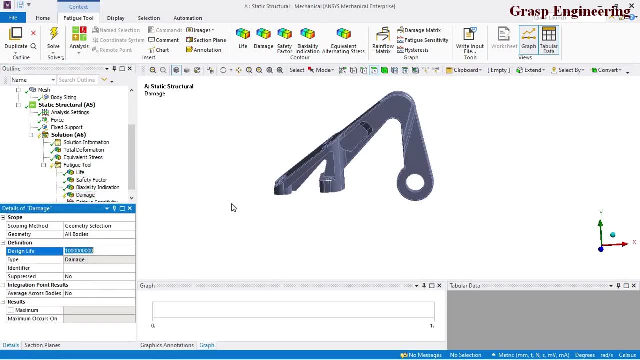 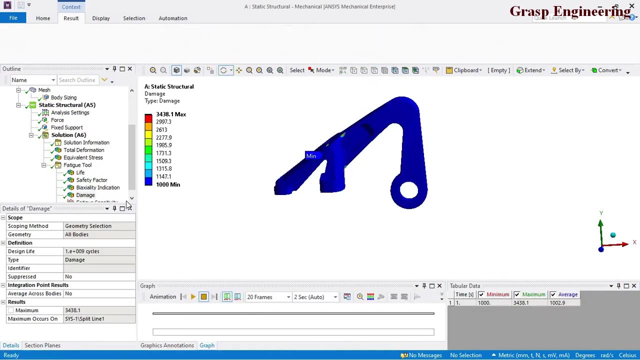 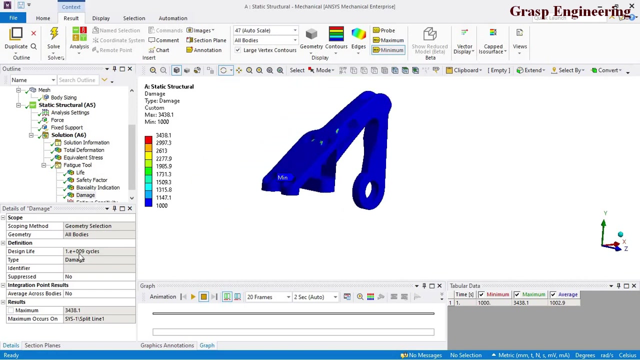 000. okay, now let's check. i think we forgot one thing. let is checking the damage. okay, now here, if you remember, our damage uh is 1.25, for which we need to find out the damage. so let's evaluate first. now, if you see that here we are getting a very much like 1000- 3000, because here design life is. 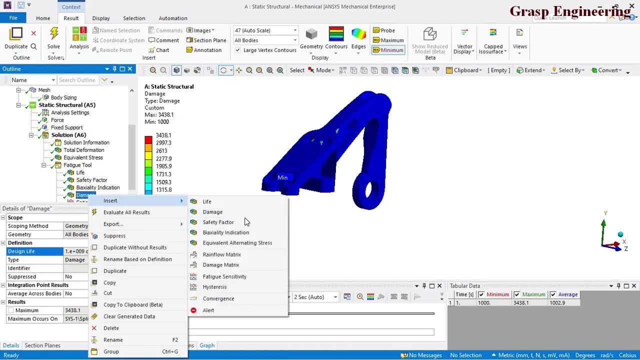 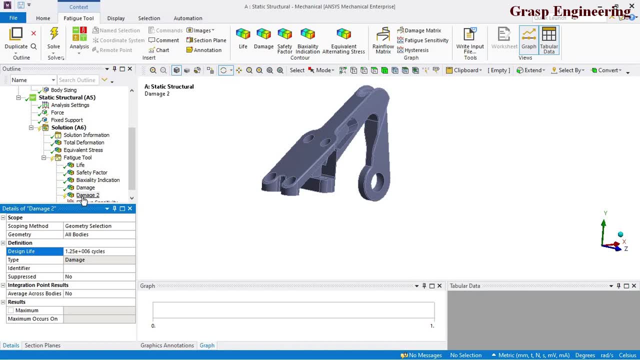 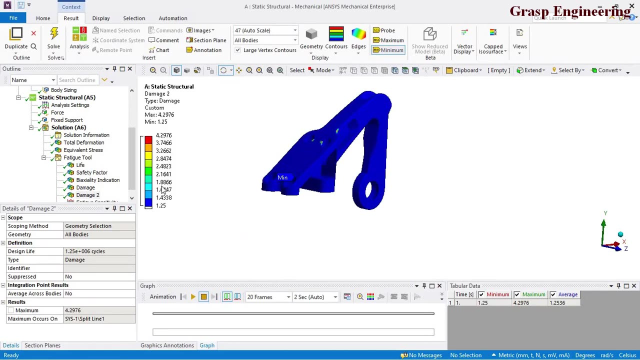 1 raise to 9, but our design life is 1.25. here is to 6.. now let's check here whether it is below 1 or not. so you can see like it is 1.2524. so accordingly, if you want to vary your design life,